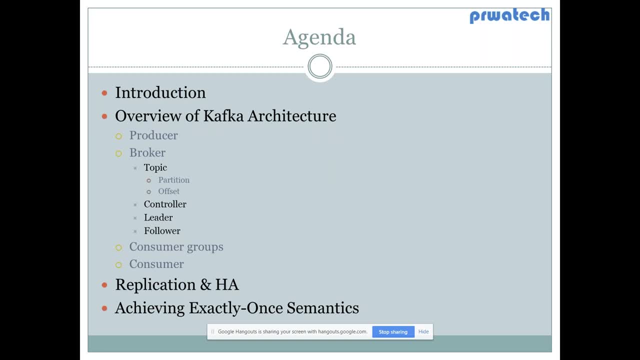 like producer, broker. So there are different parts of Kafka. So you'll have producer, then broker, then topic, the topic then partition and offset, So topic, partitions and controller, then leader and what is follower. Then we will have this consumer group, this consumer. 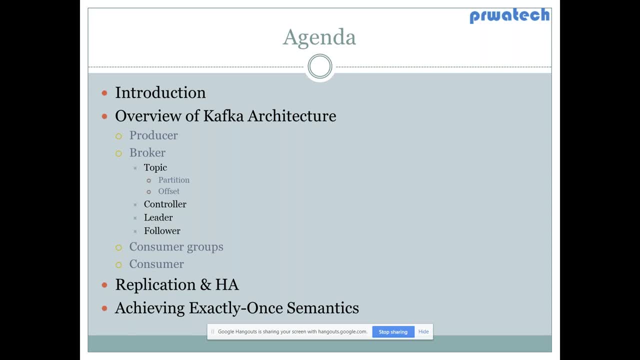 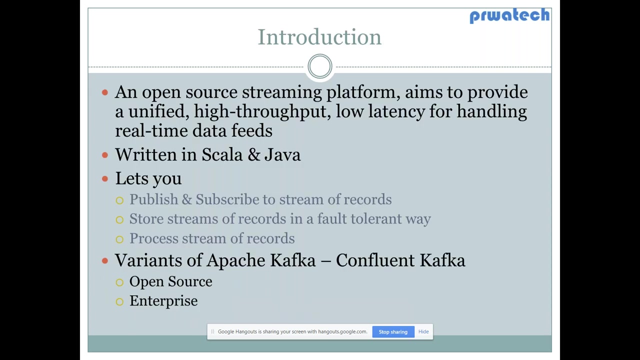 what is consumer in the consumer group? And we will know more about this application and the high availability. then we will know also about achieving exactly one semantics. So we will know. let's say one by one: so what is Kafka? Kafka is a open source streaming. 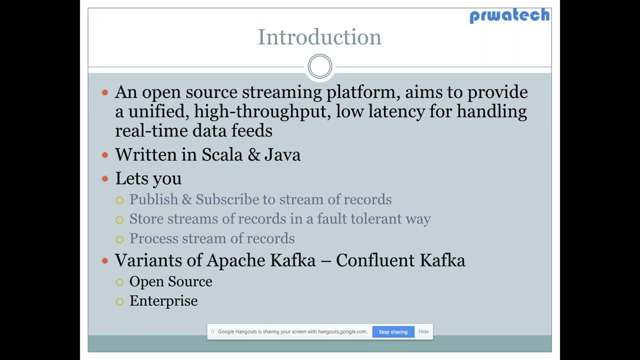 platform aims to provide a unified high throughput load of latency for handling real time data themes written in Scala and Java. So basically, Kafka will let you publish, subscribe to stream of records. then this means that there will be a producer we will go into. 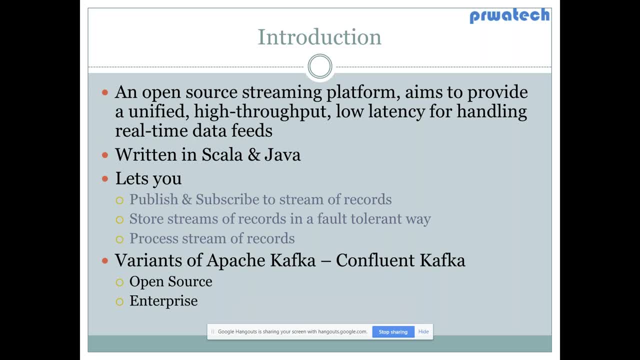 detail in the next slides. thing is this: kafka will let you publish the message and the message will store in kafka broker and then the subscriber. it can be kafka stream. must kafka consumer or any spark streaming applications which can connect to this broker and subscribe to this stream of records? kafka also store kafka as one storage api. 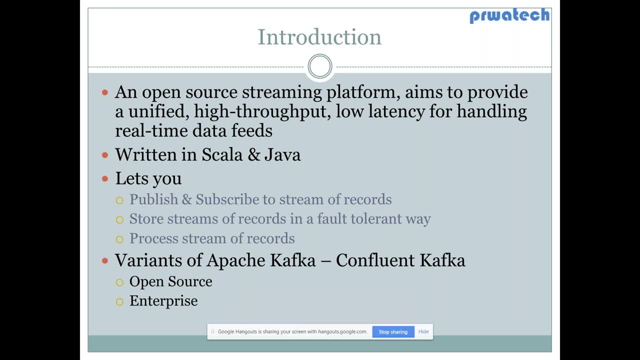 to store streams of records in a fault tolerant way then and then process the stream of records. that means in kafka stream like k stream we have. so is that? what i want to say is here is that there are many apis that kafka has, like publish, producer api, consumer api, then your stream api. 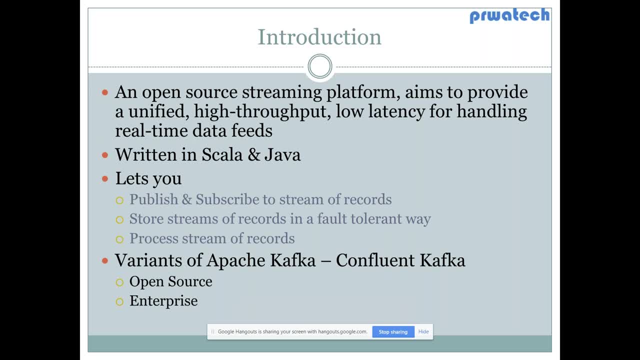 and then storage api is also there. so there are apis are there so, using which you can connect to any kafka broker and you can have an end-to-end messaging system keeping data message flow. now, talking about the value, only apache kafka is. it is the open source, it's apache licensed. then is there any other variants? yes, the 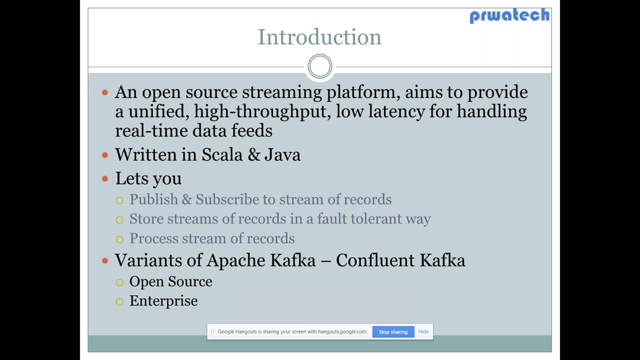 most popular variant is concurrent kafka. uh, so things that concrete kafka's two versions, like open source version is there and also there is an enterprise person. so in open source version they are providing a few features that apache kafka doesn't provide, like schema registry, and they are providing a few features that apache kafka doesn't provide, like schema registry. 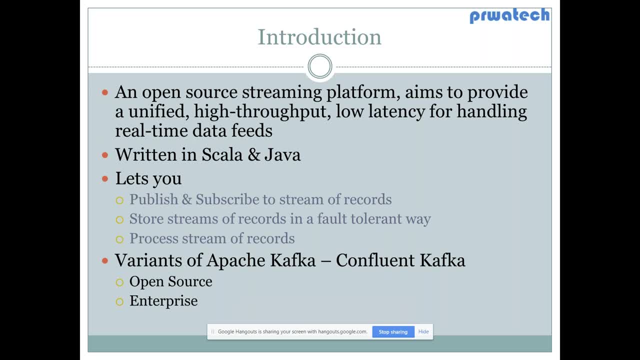 schema registry and there are few other features. also, open sources. you can try with open source. you can go to the Confluent Kafka website and can download and use their open source. now it's pretty good, and if your use case needs schema evaluation or schema registry then you can go for enterprise enterprise. 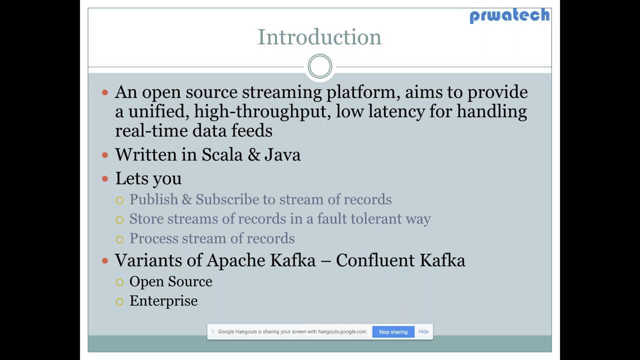 evaluation for your company thing is that you must be needing this right, so you need to have if you are using open source. also, you need Confluent Kafka support, so that would be there. but personally, you can try the Confluent open source downloading in your system. okay, so the next thing. okay, so from the 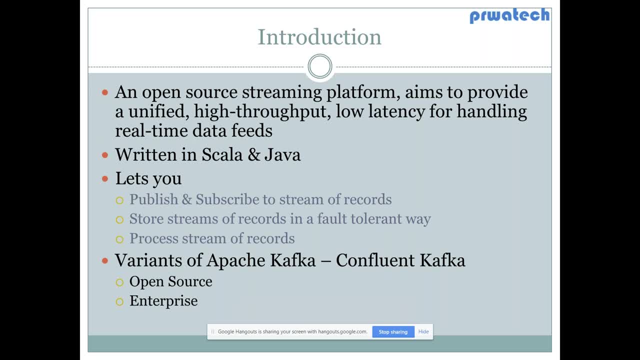 first line. what we see is that it's open source streaming platform aims to provide unified, high throughput, low latency for handling real-time data. that means it will be high throughput means there will be performance high, and there won't be it. Kafka avoids this bottleneck situations. also, like usually, it's a 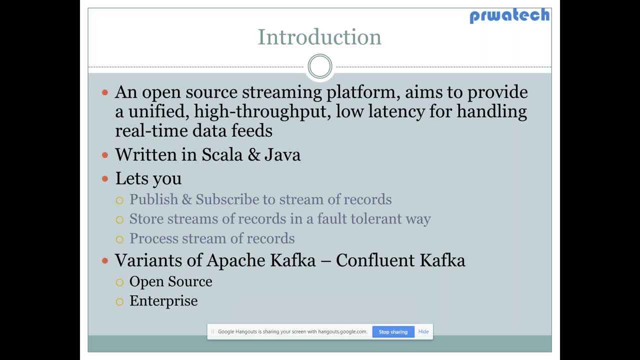 pool system. pool system, not the push system, like captive and cure. it's a pool system. school system means when Kafka will say when the producer will send the message to the Kafka broker. one is: who's push the data to the Kafka? okay, Kafka will store that. and whenever there will be a consumer ready to consume that data, that 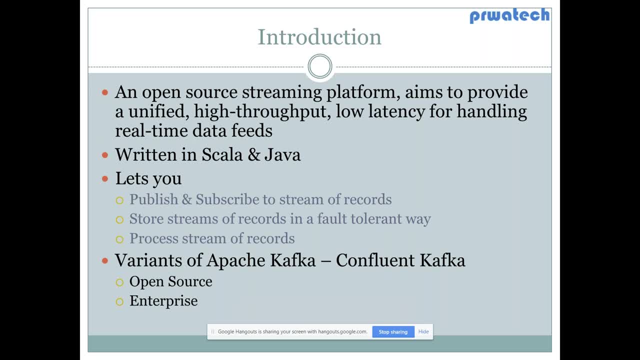 consumer can pull the data from. the Kafka broker can process the data. so there will be very less chance of bottleneck in a push system. what happens is that producer is sending a message to one messaging system. messaging system is also pushing the data to the consumer. now consumer is available or not available. if it is not available, the new. 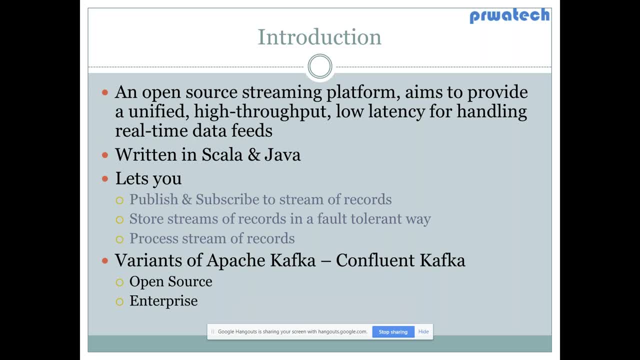 data may be lost, so push system has this bottleneck. or or if producer is sending message in large amount but consumer is not able to process that data, so in that case also bottleneck will happen. so to avoid this is the this Kafka based thought to have the retailer to have the design a school. 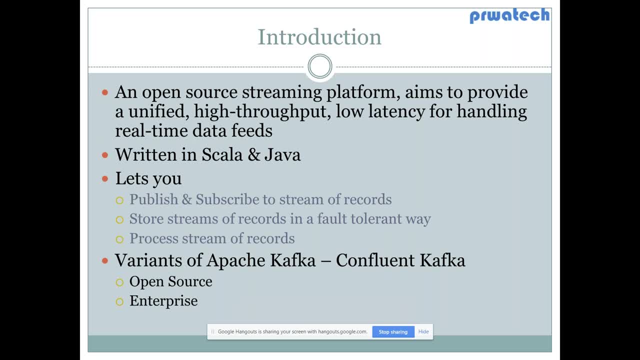 school design and low latency means it will have very less. you won't see in whenever you will get the. if you push any data to the Kafka broker in the middle, it's just you can see the data in the consumer side also. so producer will send the message to the. 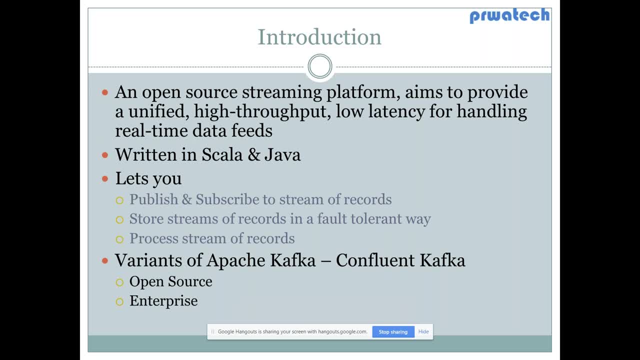 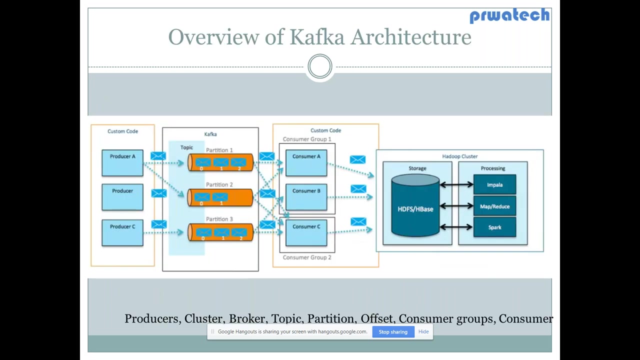 Kafka, then your consumer producer is sending message to the Kafka and then consumer is that data is available for consuming with just within a millisecond, so it's low latency. consumer is ready and you can. if your consumer is ready, then you can pull the data. okay, so to moving to the next slides is the overview of architecture, because 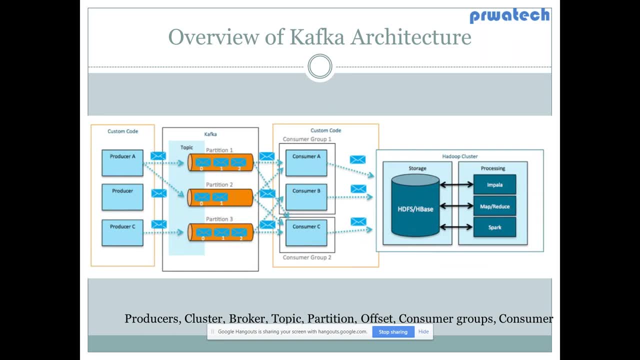 this is just a fast decision process and of Kafka. that's why I have put one slide. I have put one slide for just to have the overview, so that you will get some idea on overall end to it. okay, so this is the overview of Kafka architecture. it consists of your producer, then your Kafka broker, then your uh consumer and uh. 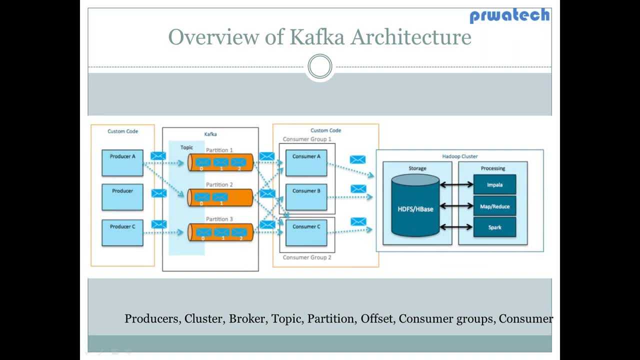 this persistence layers I have put for, like it's a end-to-end big data system, that's so. persistence is not a part of Kafka architecture. uh, it's like: uh, you have your consumer. if you can use your Kafka consumer, or you can have your Spark streaming or any other as consumer, and just okay, if you have. 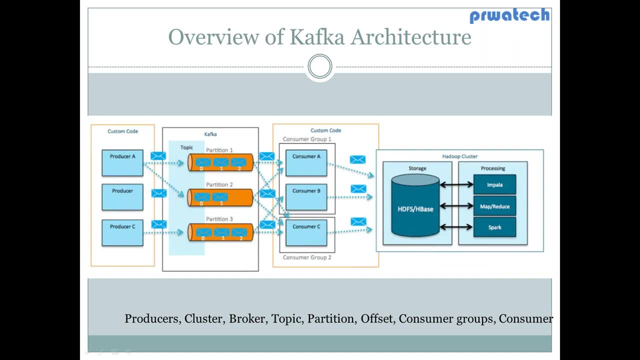 any questions? I can just uh pink to question. I will go through that at the end of this session, okay, uh or comment or anything. I mean you were getting just push your questions, okay. so the let's start from the left side is use your custom coder is for producer. now you can have multiple. 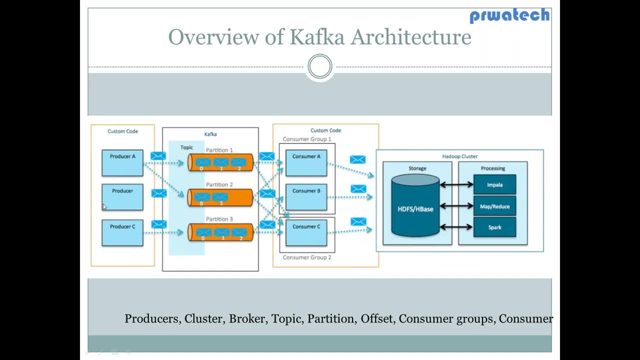 producers. if you are different, uh, like, you have retail billing, your billing, uh application, you can have your order application. or in, like, you have many the source systems. okay, so all those source system, you will get the data. you write one publisher. this publisher will push the data to. 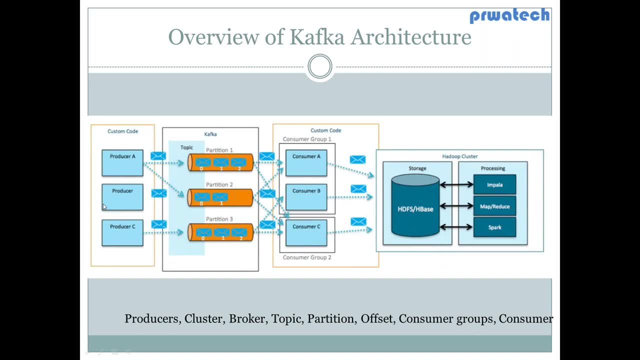 the kafka, kafka. now, uh, as i have said, it's a div type, so i will little bit uh deep dive into it. just i'm now completing the overall thing. producer. now this producer is sending, it can send to a particular topic. okay, so in that topic you will have many partitions. 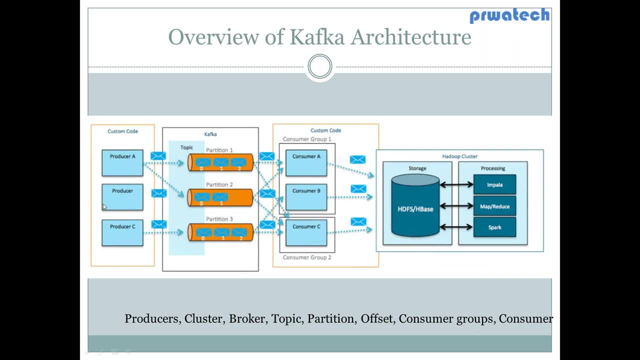 so first of all, this before that topic, you think, is that there is kafka broker or server, okay, and this broker is inside. is a cluster? cluster means number of brokers or server, okay, number of broker. now you have just, i have just the one machine, for example one, so it can it be a cluster? yes, it can be a cluster if you have multiple broker or kafka server. 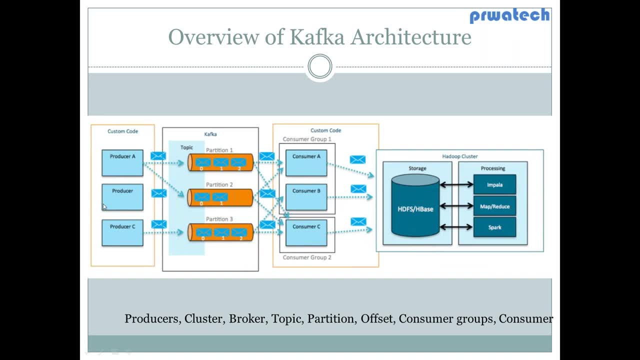 it's just alias, okay, so don't be confused. that broker is equal to some kafka server. so now if you have three, three broker inside your machine, so it's a, it's a cluster, so it's a number of broker. so inside each broker there will be a topic. 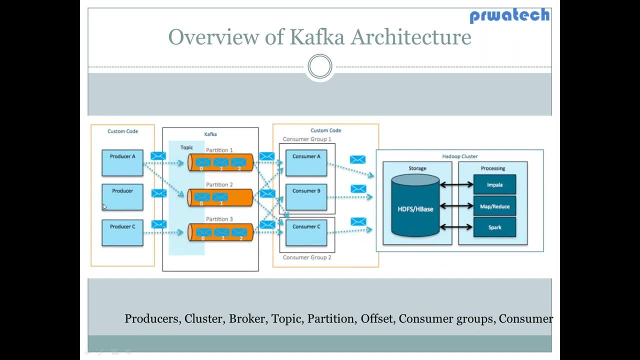 okay, yeah, not a topic. actually, you, you are creating a topic, so this topic can be in multiple broker. okay, so you, you can have multiple topic inside a broker. also. now think, is that, so this, inside that topic, there will be, uh, there will be multiple partitions and each partition in, inside each partition, your, uh, there will be a sequence of offsets. 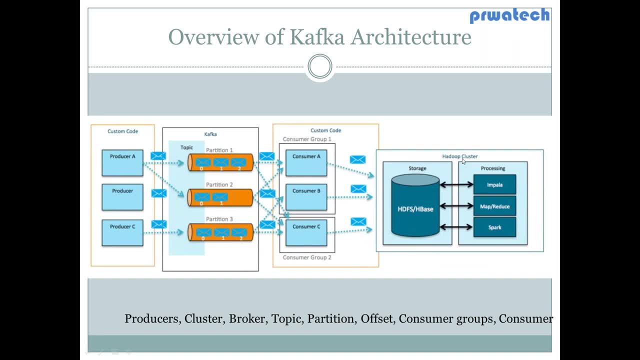 and in each offset your message will be stored. now this producer knows to which topic it is sending your time, sending the time, so it will, while publishing, it will mention that, okay, this topic. i want to uh to publish the data and. and it can mention the partition or there is a default partitioner also. 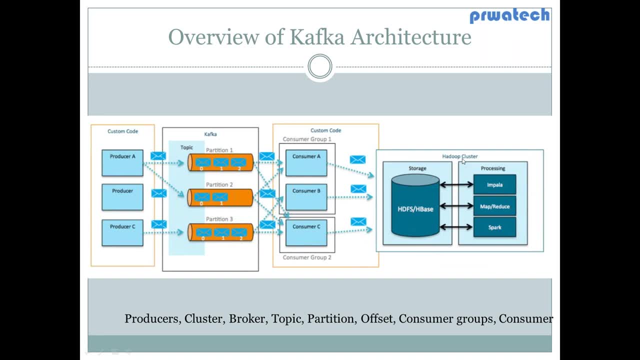 so when this message will come from the publisher to the topic, now that in the now this message. as for the key, the message will be divided into. well, the message will be: uh, pushed to particular partition, okay, uh, okay. so i i don't want to confuse here thing, is that? so let's, let's. 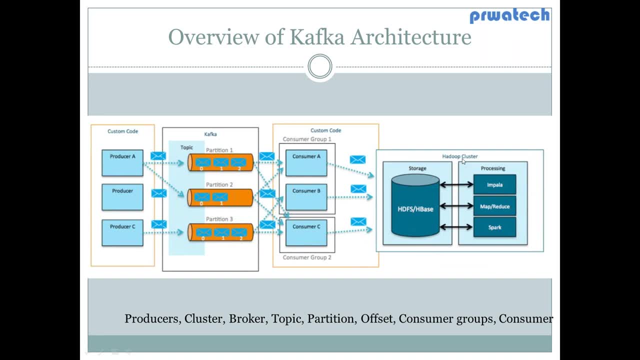 have just one flow. the producer is sending the message and messages are residing the inside the partition and from the partition consumer can read from the multiple topics as well. so consumer can mention, mention which topic it is trying to read data and it can read the messages from the. 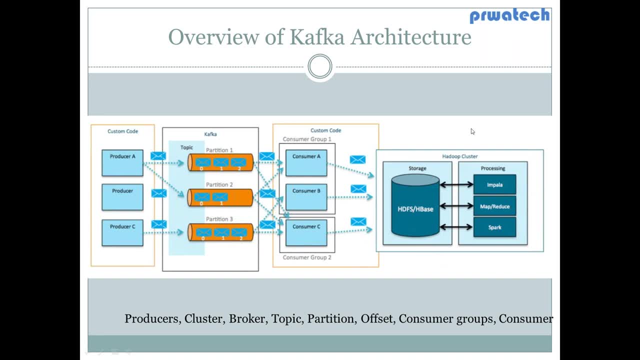 partition. okay, and why in this custom put this custom code means: uh, this consumer said: this consumer can be your kafka consumer. okay, stream, kafka stream. and also it can be your spa streaming application. when it gets the data, it will. you can do anything in any, any manipulation. 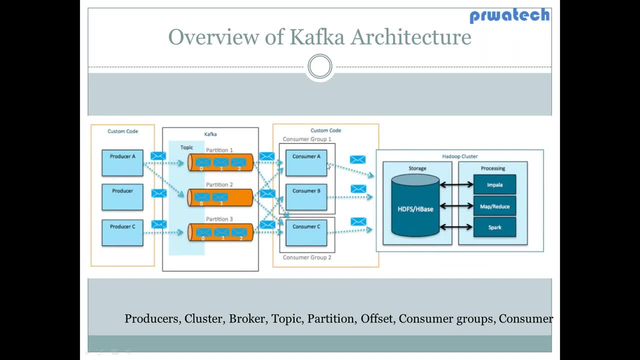 you orän your transformation and store it anywhere- hdfs, hvies, hype or something like that? okay, uh, kafka have its own storage or it's using hdfs or hyIPs for store tata, okay, so to answer this question. uh, higher sunoo. uh, so to answer your question. actually, kafka is also on your. 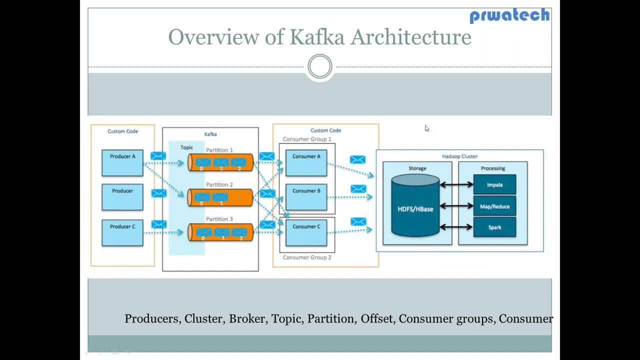 local or you on your file system, like unix file system. okay, so you can mention the hdfs location also to where your data will be stored. that will be hdfs, but by default it is stored, uh, in your logdir property in your serverproperties. kafka has the serverproperties in the conf folder there would. 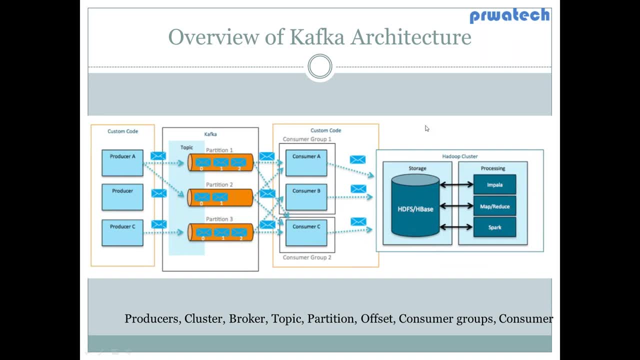 be logdir configuration there. the usually the default value is tmp slash. tmp slash- kafka hyphen logs. there, actually, your data is being stored in each partition where data is being stored inside your partition, right? so there will be multiple files like topic, topic name, hyphen, uh or underscore. 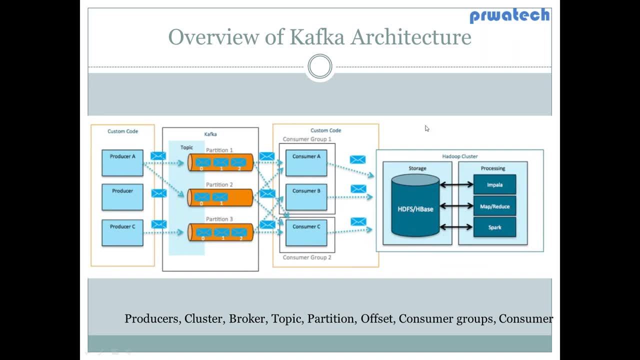 like topic name underscore your partition, partition id. okay, each, each partition has its id. topic has also id. so like topic zero, partition one, and inside that there will be two files. there will be one index file and another will be your data. okay, uh, so i think this is this answers your question. we will discuss into it. i will deep dive. 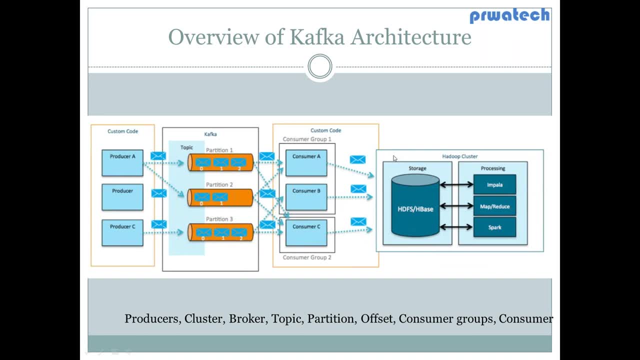 okay, so we will discuss, just to have this now. can multiple producers send data to for same topic? yes, sir one. yes, uh, multiple producers can send data to a, uh, to one topic. thing is that, uh, when producer sends data, it mentions the topic in the publisher code. so your multiple producers. 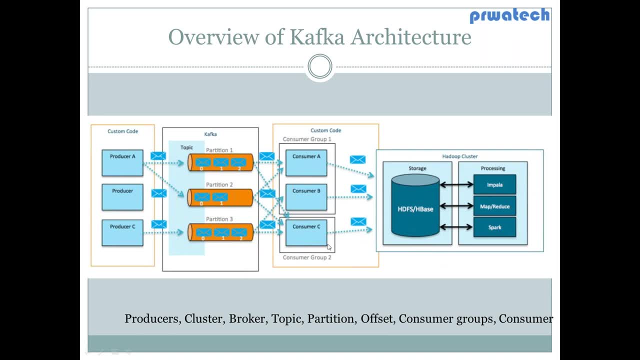 can send this, uh send like: your billing system is there, your order system is there, payment system is there. so multiple source system. they want to uh. they want to uh push the data called a trade topic so all they can store in the trade topic. i'm not telling about design perspective. what will be the best way? 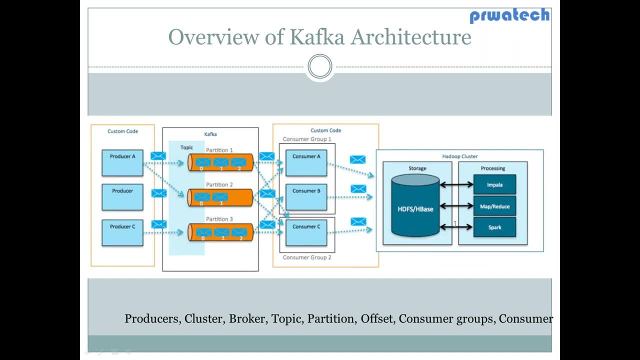 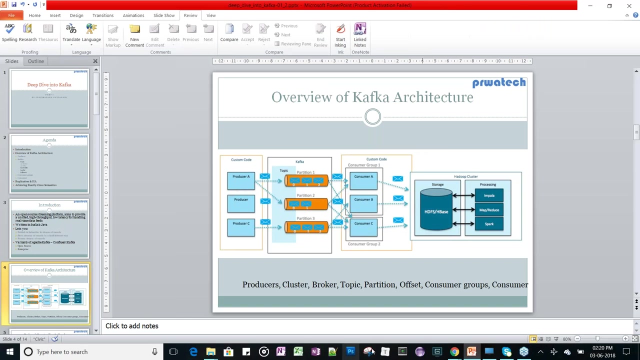 but, yes, multiple producers can send the data to the same. okay, okay, uh now, um, okay, before going to the next slide, uh, okay, so let me uh a little bit deep dive here. so what i will do, i will draw, because these things will explain in the faint way. so 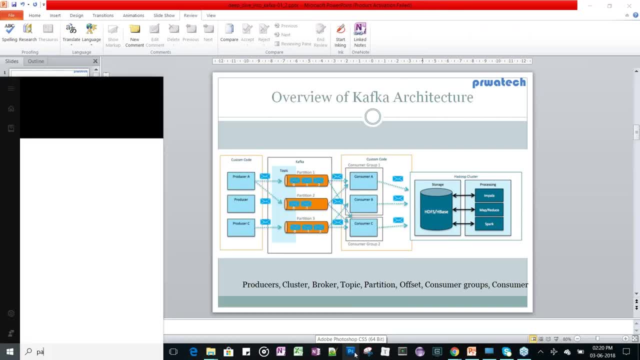 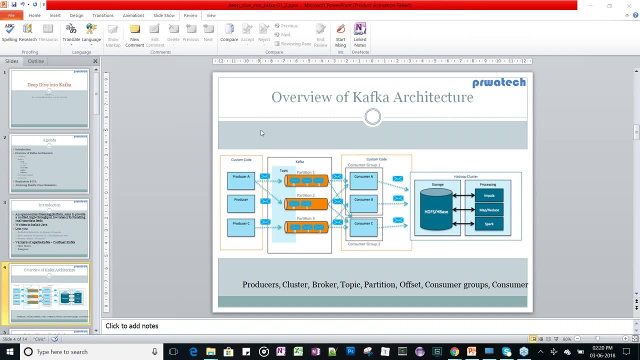 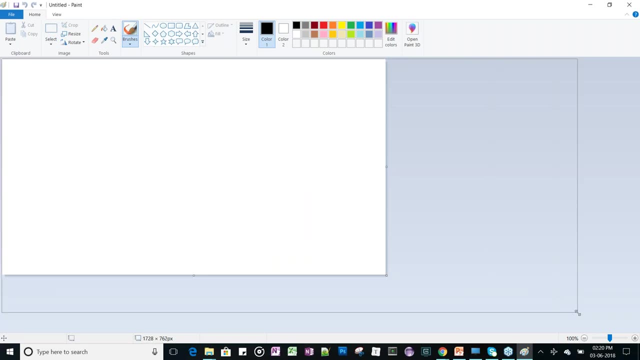 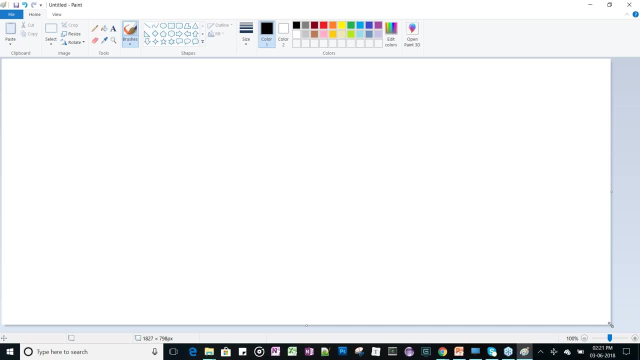 that, uh, let's see from the publisher side. okay, so, this is your publisher. you can, uh, you can send um this inside this publisher, you can. okay, so, each record, uh, inside this, this is one publisher p1. okay so, publisher, so each record, uh, you can push and let's have. 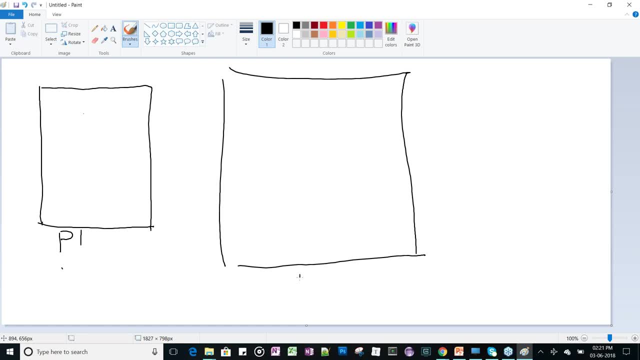 this is kapka. okay, this is your kafka broker. so, uh, each record you can send or you can post it inside the share, your website. you make a batch, batch of record because if each record you want you have to send to broker, there will be a much network input, output, network flow. that is also 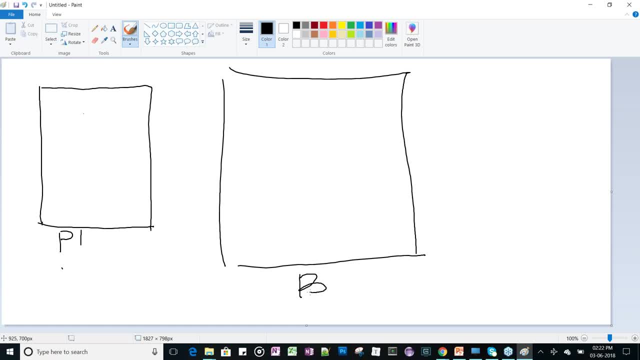 bad thing. so what we will have? we will have a patch so you can have, let's say, actually this: whatever this record in the message in the publisher, we will call it producer record. okay, producer record. in this producer record, there there will be your topic name, topic and then partition. then what's your key? 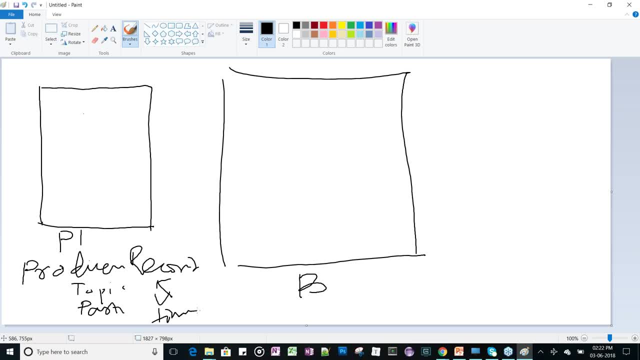 value and timestamp. key me there in in your message. okay, in message your message: your key value and timestamp key in your message. okay, in message your message: your key value and timestamp key. there will be a key you can you can make. there will be a key you can you can make. 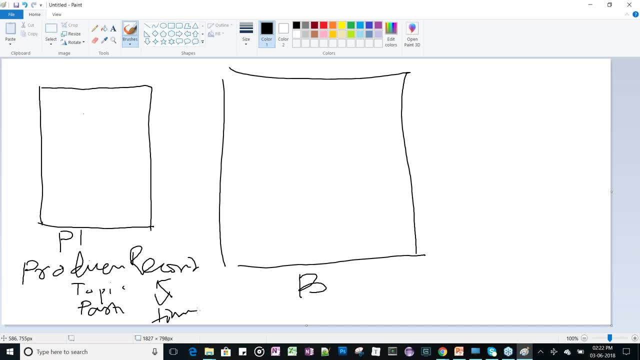 there will be a key. you can, you can- make your what will be your key, and then the your what will be your key, and then the your what will be your key, and then the doorway value, now this. that means this. doorway value, now this. that means this: 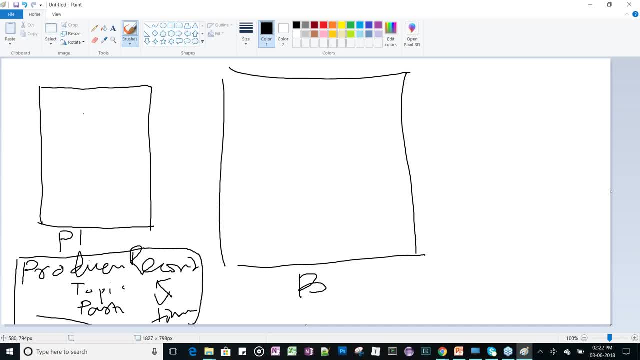 doorway value. now this. that means this producer record contains this five producer record contains this five producer record contains this five information topic: which partition? key information. topic: which partition? key information. topic: which partition? key value times: now this partition is a value times: now this partition is a. 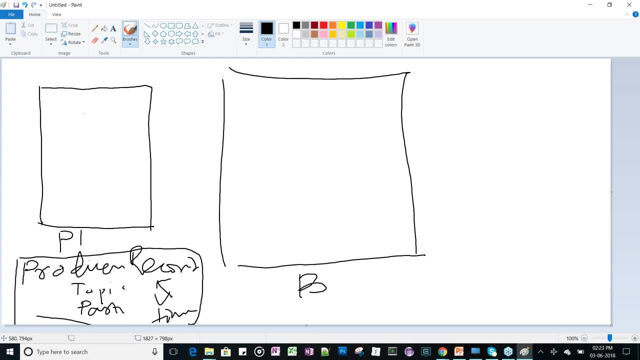 value times. now, this partition is a little bit problematic, right so, which little bit problematic, right so, which little bit problematic, right so which partition. I don't know so what I will do partition. I don't know so what I will do partition. I don't know so what I will do to the produce, or what I will as a 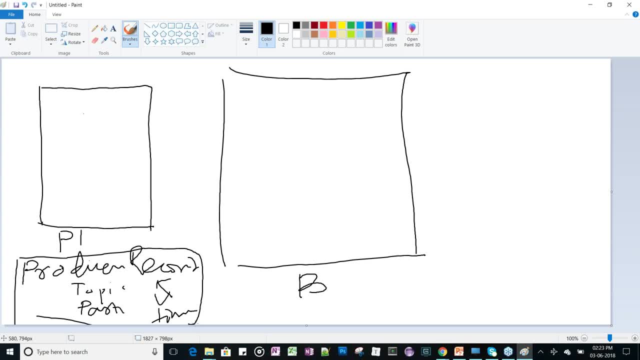 to the produce, or what I will as a to the produce, or what I will as a producer- what I will do, I can mention. I producer what I will do. I can mention. I producer what I will do. I can mention. I can keep it blank like I don't mention. 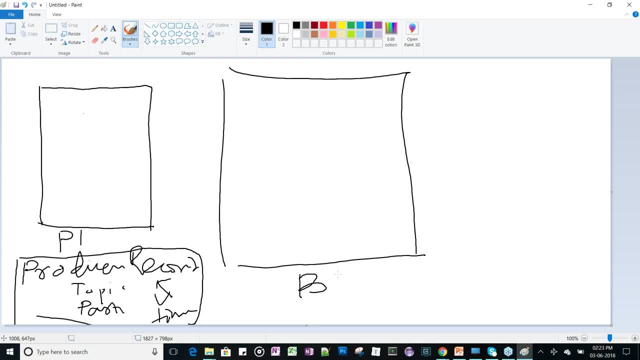 can keep it blank like I don't mention, can keep it blank like I don't mention any partitioner. in that case, it will be any partitioner. in that case, it will be any partitioner. in that case, it will be a default partitioner. okay, so if you. 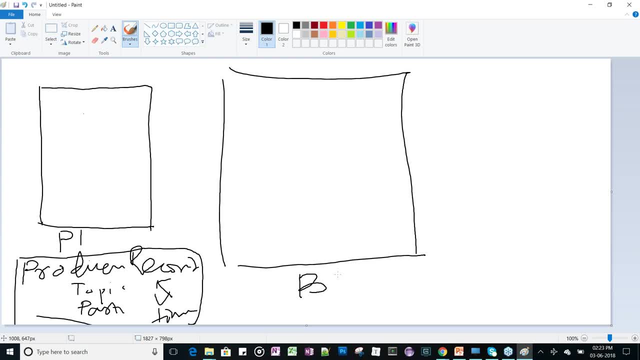 a default partitioner, okay. so if you a default partitioner, okay, so if you have any partitioner, because if you have have any partitioner, because if you have have any partitioner, because if you have any partitioner, you mentioned that, so any partitioner, you mentioned that. so 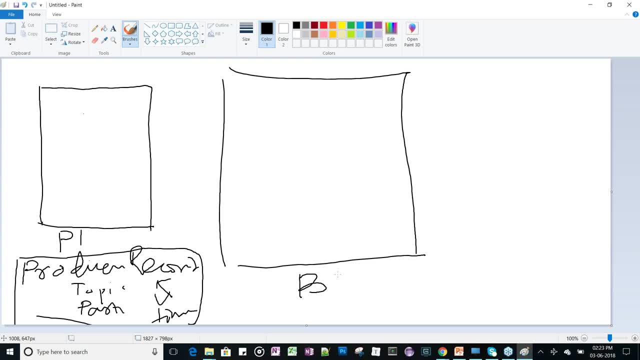 any partitioner. you mentioned that, so that will be direct, that's called direct. that will be direct, that's called direct. that will be direct, that's called direct strategy. if you have, you don't have in strategy. if you have, you don't have in strategy. if you have, you don't have in mention any partitioner, then it will it. 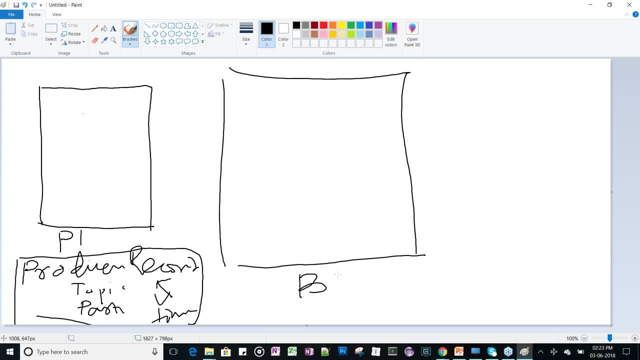 mention any partitioner, then it will. it mention any partitioner, then it will. it will be default partitioner then. if you will be default partitioner, then if you will be default partitioner, then if you have your key as the partition strategy, have your key as the partition strategy. 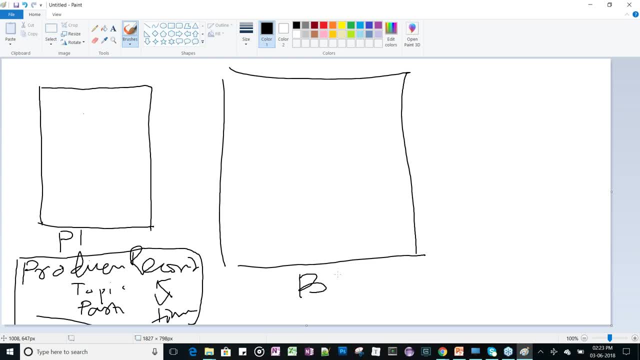 have your key as the partition strategy, then it can be your key module using, then it can be your key module using. then it can be your key module using your key. it will decide which partition your key, it will decide which partition your key, it will decide which partition, which partition inside that broker like 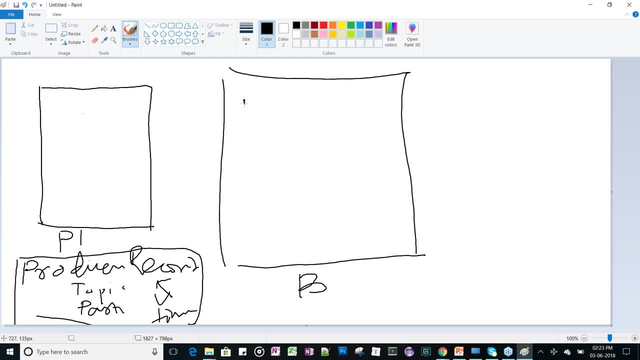 which partition inside that broker. like which partition inside that broker, like inside this broker. there will be a inside this broker. there will be a inside this broker. there will be a topic here, okay. so let's say this is, let's say this is one topic and inside. 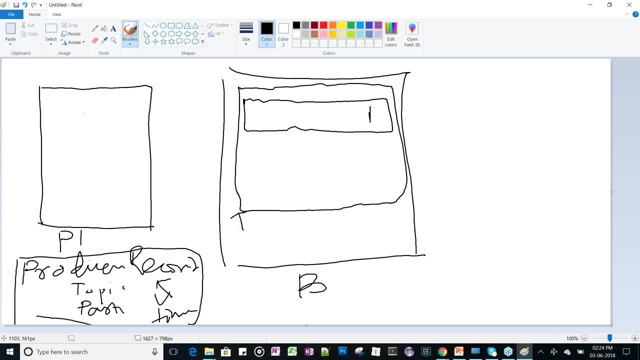 let's say: this is one topic and inside, let's say this is one topic and inside that topic, if there is a partition one, that topic. if there is a partition one, that topic. if there is a partition one, zero and there is a partition, so now zero and there is a partition, so now. 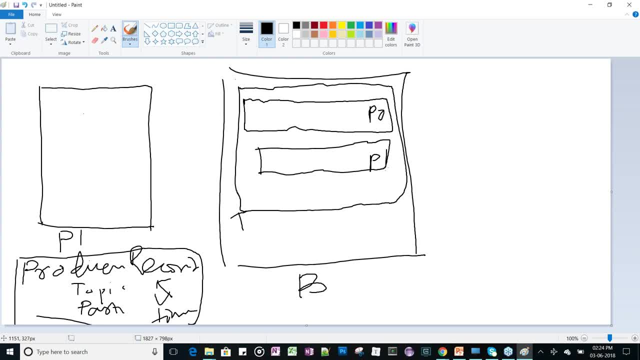 zero and there is a partition. so now, this you can mention like in your key. this you can mention like in your key. this you can mention like in your key that which partition you should go like, that which partition you should go like, that which partition you should go like. ask for your key, either that that will. 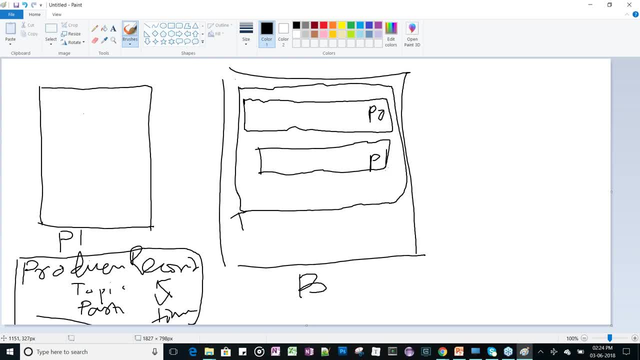 ask for your key. either that that will ask for your key, either that that will be key modulo partitioner, or you can use be key modulo partitioner, or you can use be key modulo partitioner, or you can use your custom partitioner. so, if you are, 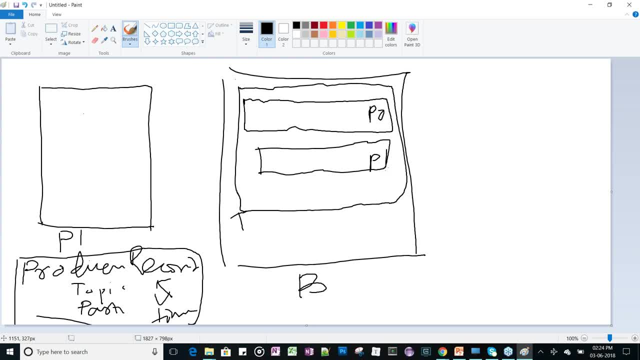 your custom partitioner. so if you are your custom partitioner, so if you are using custom partitioner, then according using custom partitioner, then according using custom partitioner, then according to your algorithm, it will select which to your algorithm. it will select which to your algorithm. it will select which partition your data should go. so topic: 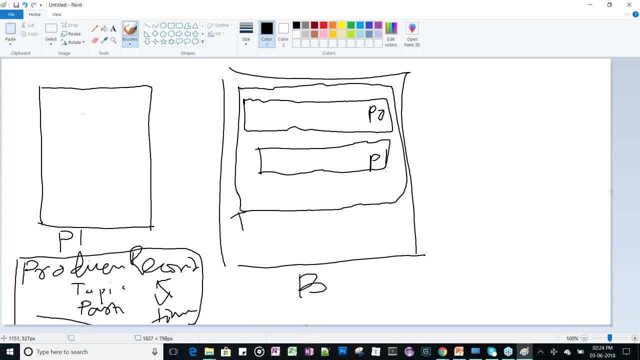 partition: your data should go so. topic partition: your data should go so. topic is mentioned from the producer side. is mentioned from the producer side. is mentioned from the producer side. partitioner is calculated now, before now. partitioner is calculated now, before now. this: after selecting the partitioner, it will also serialize your data, so there. 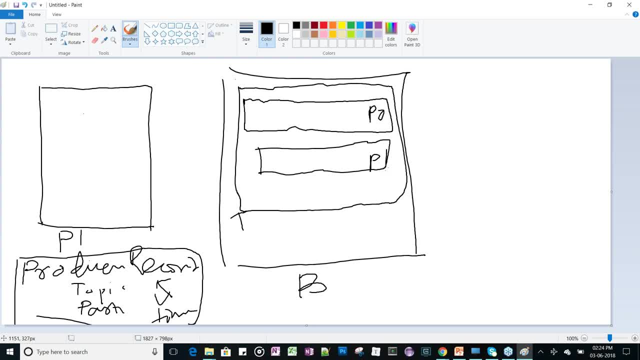 will be in the producer side. so this producer record will be there and this partition will be decided. then serialize, which serializer you should use, that also being decided, and after that your record will go to the will go to the broker. okay, so this serializer also, you can have your a gross serializer, you can. 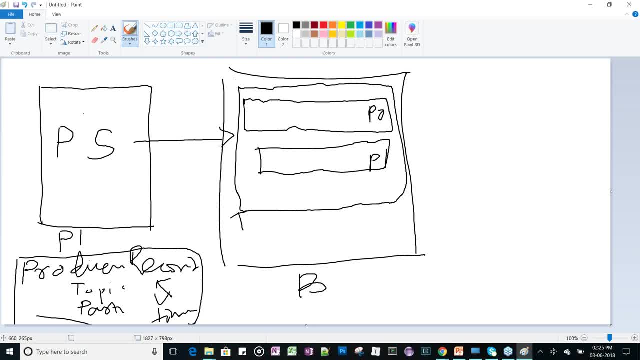 have a pro is the default serializer for Kafka and you can have custom serializer also, Java serialization also you can use, but that is a bit heavy. so what do we use? is a pro? mostly so- partitioner, then serializer, then okay, so now each record instead of sending each. 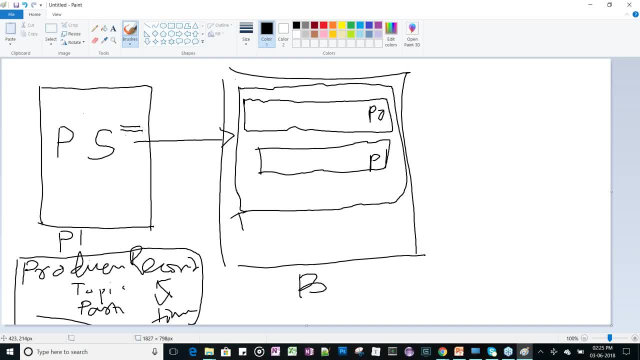 you record. you can have multiple record clubbed together, so it's called batch, each batch. okay, so there will be multiple record called batch. so you can, you can send in batches. so what? what in you to? what you need to mention is that your memory buffer okay. so, for example, your, you have decided your memory buffer. 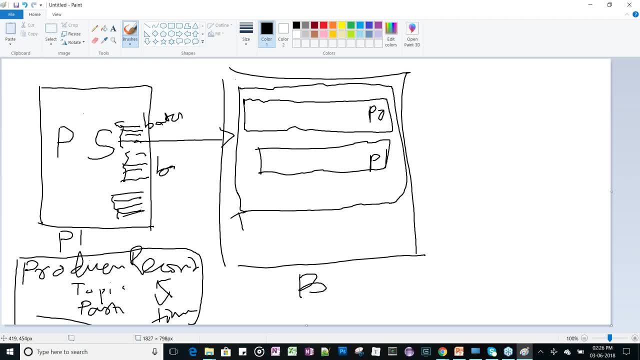 at 64 kb. one in the site, so in 1, or 1 in the, for example, one so in one MBE. you can mention your batch sites each, how much. that is all configuration so like how much you will be your bad sage and how many you how much will be your buffer sites, so in a 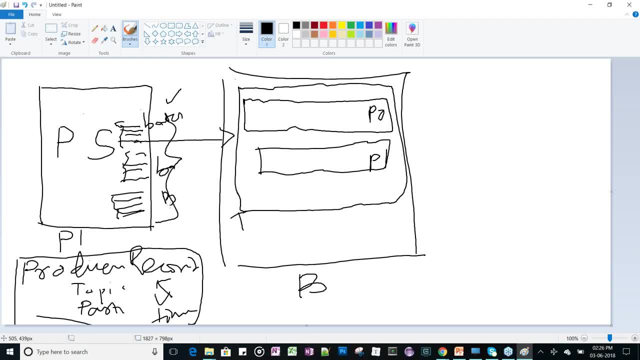 buffer, there will be multiple patches and this whole thing can be serialized in. it can be also compressed. also, if you want to decrease this network bandwidth, you can compress it using snappy or zzip or lz, so you can uh compress it and the data inside the data will. 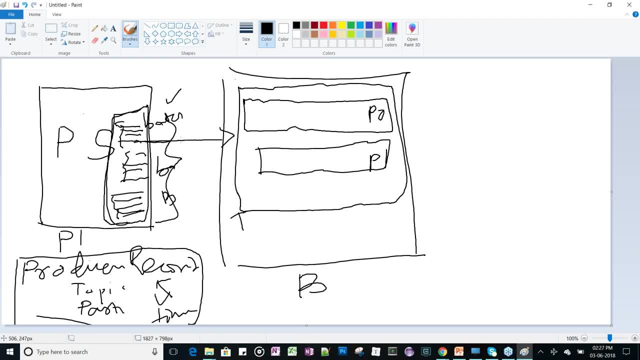 be serialized. that will be passed to the broker. inside the in in the broker you decompress and deserialize and then you process your data. but think is that the only problem here is that there will be more cpu processing. okay, so, depending on uh, your use cases, like you, if there is more cpu. 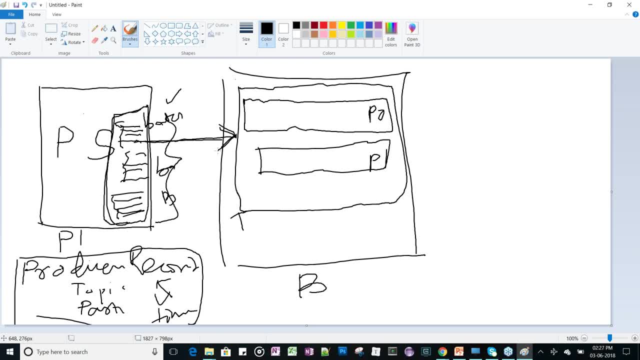 intensive operations can handle, then you can go through this, or you can simply: you can have your abro serialization- uh, no need to compress you. just you have abro serialization and use batches for sending the data from producer to broker. okay, so inside this broker, inside this, this is kafka. 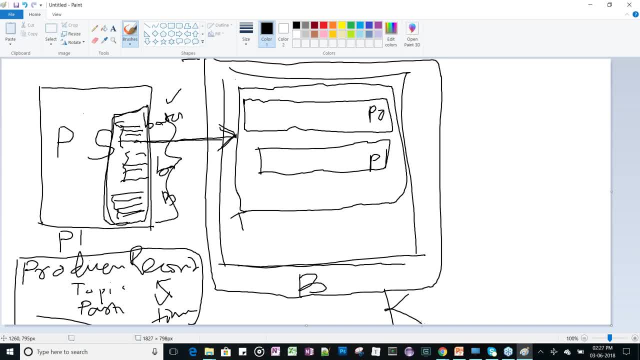 cluster, big one, this is kafka cluster. inside that there will be many broker and each broker will contain many topic. will say: one topic here, okay, and inside each topic there will be multiple partitions, so it will go to the each partition and each partition there will be a offsets. 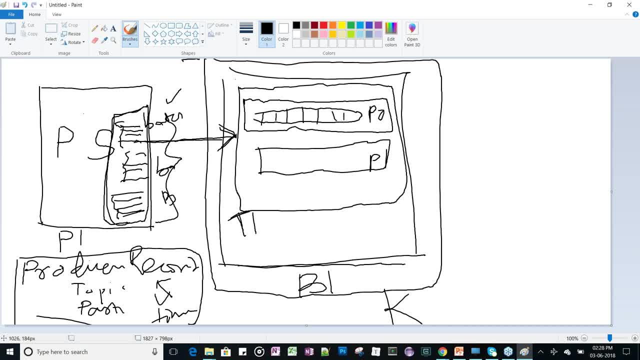 okay. so in kafka language you can, uh, you will see in the document log, log is nothing but your, uh, your, your each partition, okay. so there is a concept called log compaction. that is nothing but your partition compaction, okay. because in log, when you, when someone says log we, we understand. 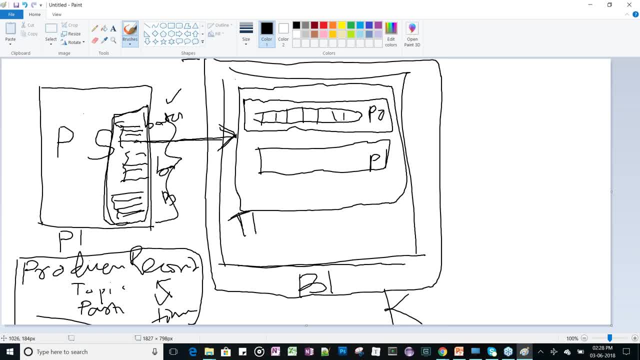 it's a logging or something somewhere. so in kafka we log for log as like you can consider as a partition. so, uh, so, in each partition now there will be many scenarios and all this. okay, we'll go one by one. let's first let's understand this: publish to some. uh, partition, uh, publish to. 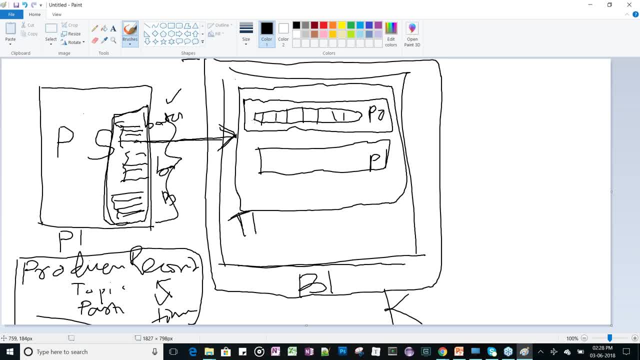 publisher to kafka. now we will go to inside kafka broker. so we'll see. okay, so there will be multiple partitions, um, and okay now. uh, now we can go to the consumer side. okay, so in this consumer side, what can happen is that, uh, this consumer can be your kafka consumer or it can be a spark. 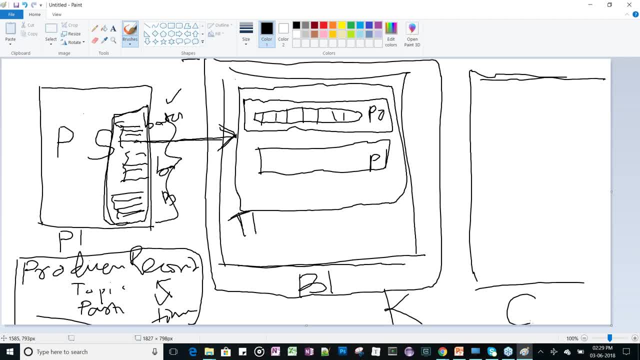 streaming application. okay, so this past streaming application also. you need to mention which topic, which topic you want to uh listen. okay, so you can also mention, like, how many trade will run also, uh, but which topic you need to mention in your consumer consumer now, from the kafka perspective it is, your consumer is divided actually. 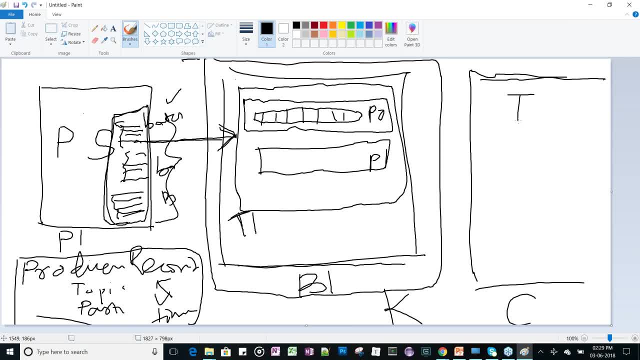 it has consumer groups. it divides your each consumer into like. what i want to say is that there will be multiple consumer group. let's not have this. let's call it cg, okay, consumer group. this is one consumer group. there can be another consumer group also. or let's divide, like. 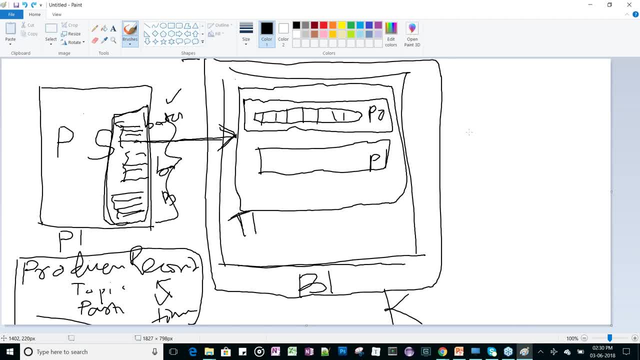 this. so let's have two consumer group. this is cg1 and this is cg2. okay, i divided into two consumer group to just show like how things are working. consumer: you can uh say like there are multiple applications, you, you have this kafka unified message messaging system. 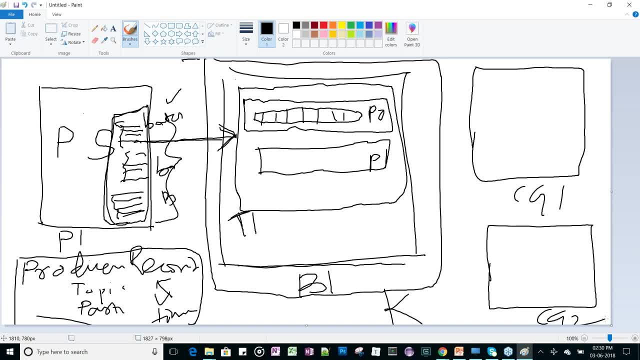 now you have multiple applications. okay, your, for example, billing system has a different application, your another. some data lake system is also there with data partner, data scientists, data science guys are also there. so there are different consumer groups, so inside that also you can. you can have multiple consumers. this consumer is nothing but your. uh, when you say: 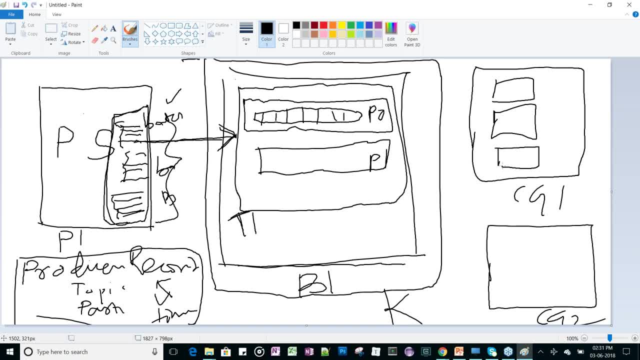 in the spa streaming. you need to mention that. okay, local to, or how many consumer thread you want to run, you can imagine that. so there will be multiple consumer. okay, but in consumer group or, for example, let's think about: uh, like this is one i am running in eclipse, this. 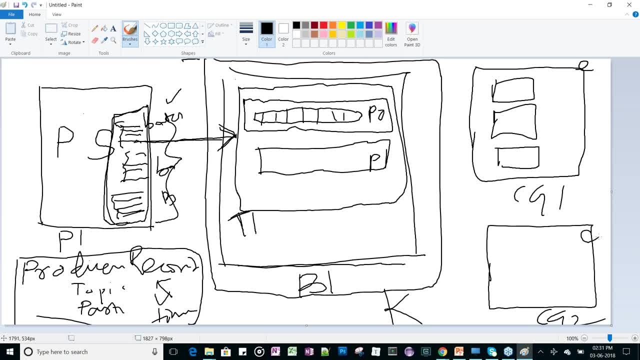 application and this is i'm running in your console, this is your console consumer and this is your eclipse or intelligent id, any ide consumer. so inside that, in in the ide consumer, i am running one spark streaming application and i have mentioned that. okay, local three, local three. 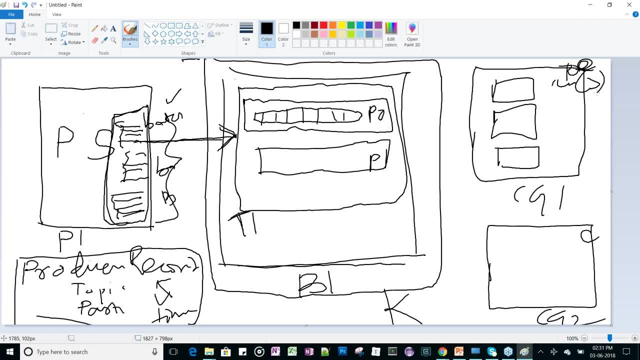 three thread will, which will run, and it will connect to this topic. i need to mention in the establishment which topic you want to uh connect. so it's connecting to this topic. now, kafka, what it will? it will connect to topic and pull your data. this is a pull system, right? so? 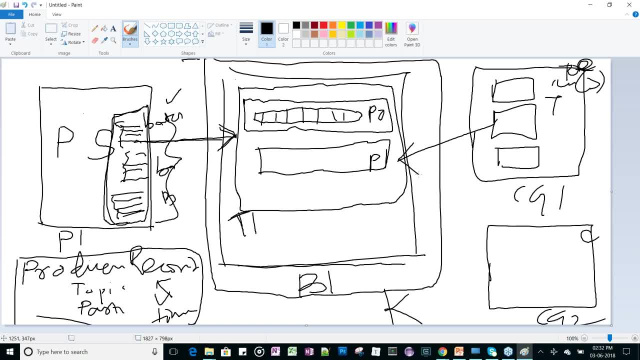 now, uh thing is that the rule is each partition data will go to each consumer group. so this consumer group, this partition is going to this consumer group and this consumer group. okay, the same partition messages, uh, same partition messages will not go into multiple consumer in a consumer group to. 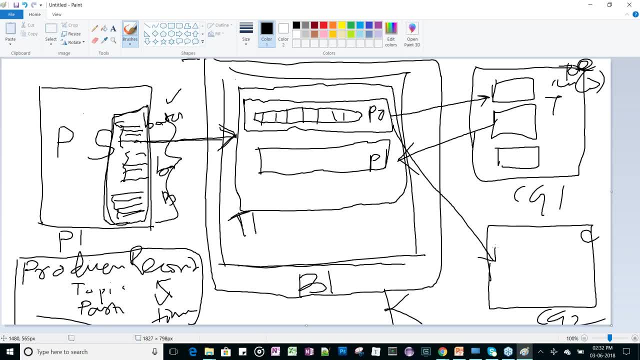 block your uh. why it is like that? just to duplicate processing. okay, so you will have multiple. so this p1 is also there. so p1 will go to another consumer in your consumer and here it will go to this one. so here, for example, there is only one consumer. 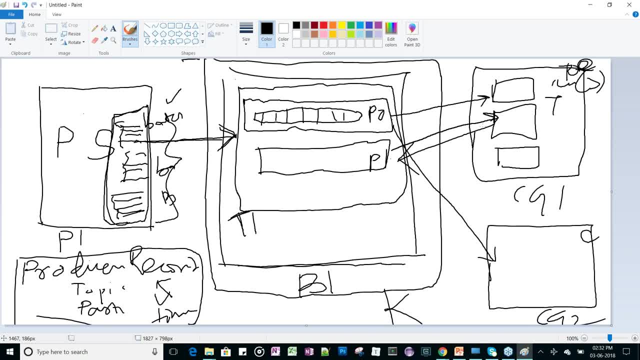 okay, so this is one consumer. so p0 is getting uh, cg2- this one consumer and p1 was also being pulled by this same consumer. but in case of consumer one, p0 is being pulled by one consumer of consumer group one and another consumer is pulling another system and this becomes ideal: another, another consumer. 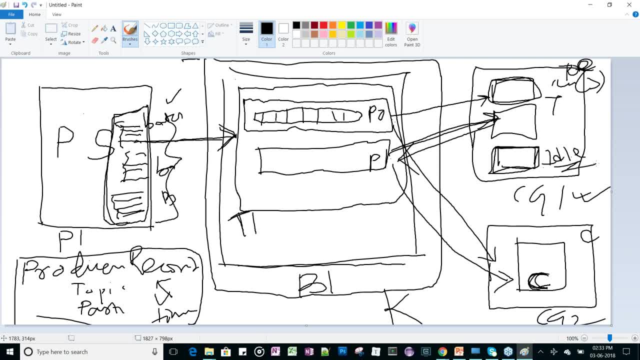 that another consumer you have created is the ideal. so your parallelism depends on, like, how many consumer you have and how many partitions you have. you know, Kafka broker, you can, you no need to have more consumer than your partitions in your Kafka. as you see here, this becomes either this consumer, this consumer is. 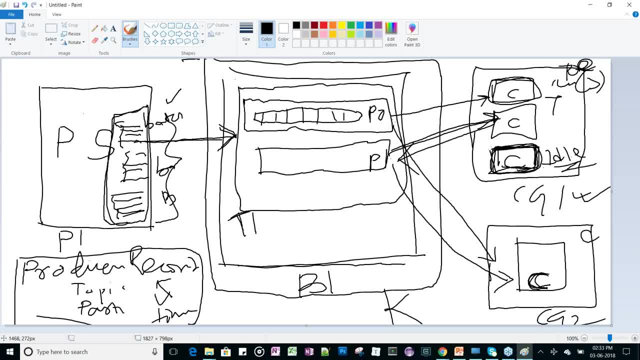 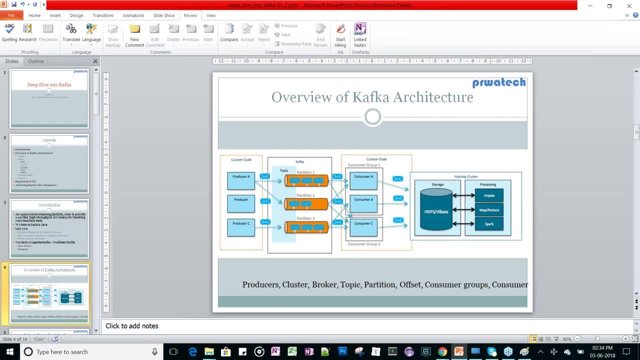 becomes idle. okay, so, okay. so. we discussed about producer, we discussed about cluster number of broker. that means then we decide a broker. that means then we decide a broker. that means then we decide a broker. that means then we decide. we discussed about topic. a topic is the unit of Kafka. so and then? 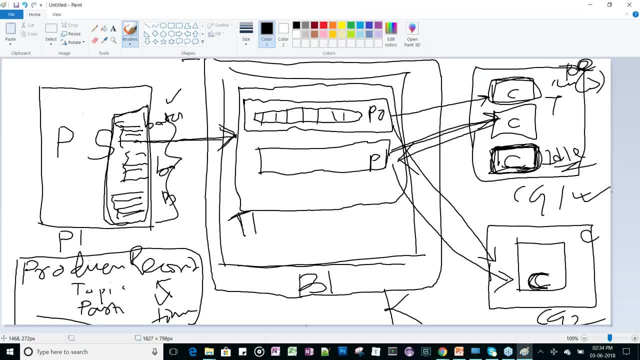 partitions. then we decided: offset. offset is nothing but your inside this partition. the messages are stored sequentially in order manner: okay, zero, one, two, three, four, five, six. in this like offset, these are offsets and this is in or in order, whatever the message we are. the thing is that so we will, for example, dispatch: okay, this batch one record using this. 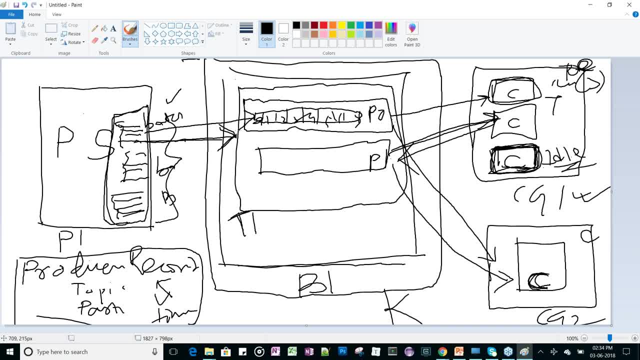 partition, partition or the logic went to this p0. another report went to the p1. okay, like that. okay, for example, it happens like that, so fast I could, went to the 0 offset and here also there will be an offset in the p1. and another record went. 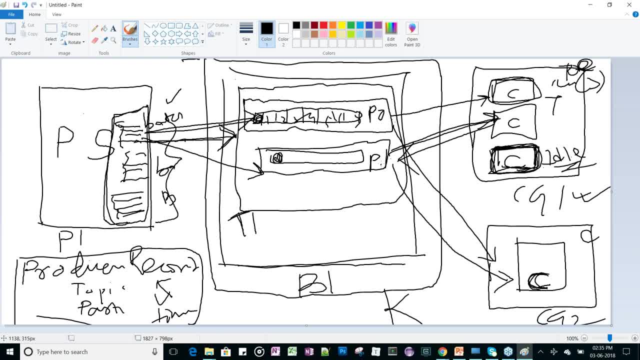 to the 0 offset of second partition. third record went to the first uh index of the first one, one index of p0. like that thing is that as a total it is not ordered. order is maintained only at partition level. only at partition level you can get the order. so if, if your requirement is that you need to maintain the order throughout, 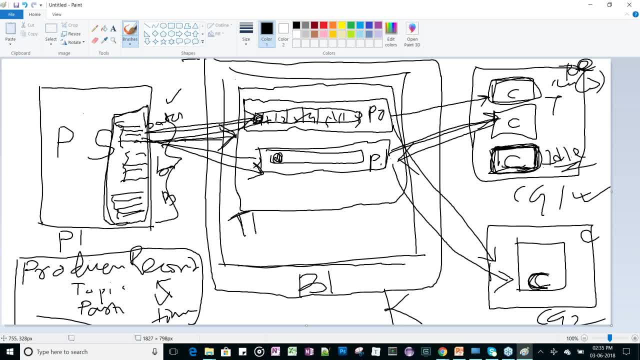 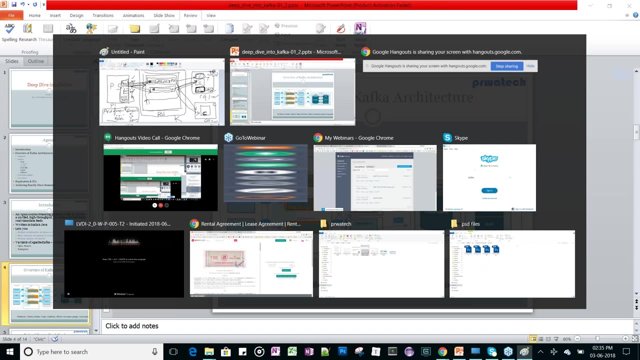 your application. then you then there is a limitation in kafka what you can have in your design that you can have only one partition in your topic. okay, so if you have one partition, then your whole data is ordered. this is the limitation in kafka, okay so? uh, then we discovered there was consumer groups. 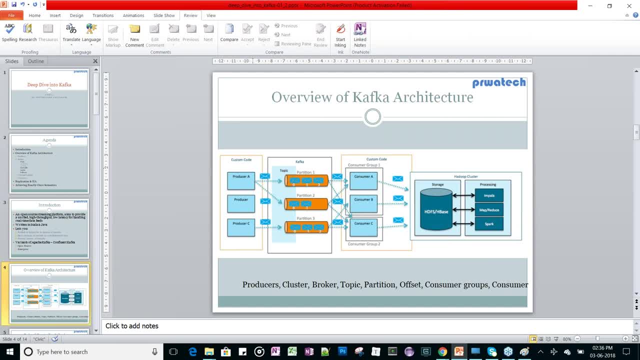 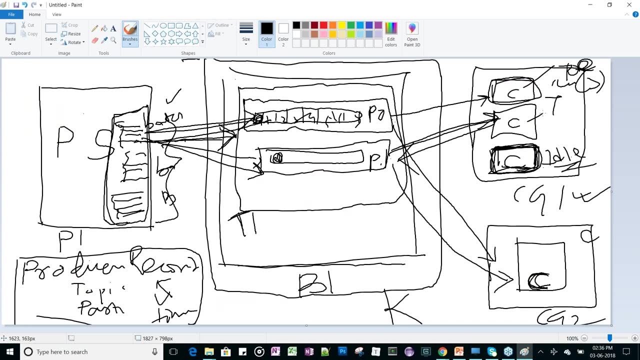 okay, which consists of consumer and who decided consumer. so it is, each are is consumer and this partitioning is for parallelism. like there are two partitions, so only two parallelism can can happen. it can be, uh, achieved if you have multiple consumer. that doesn't mean that your parallelism will increase. 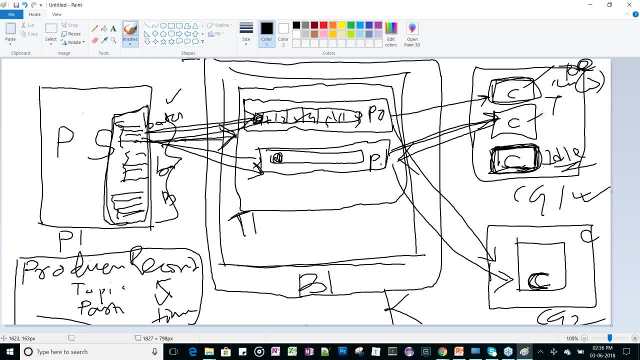 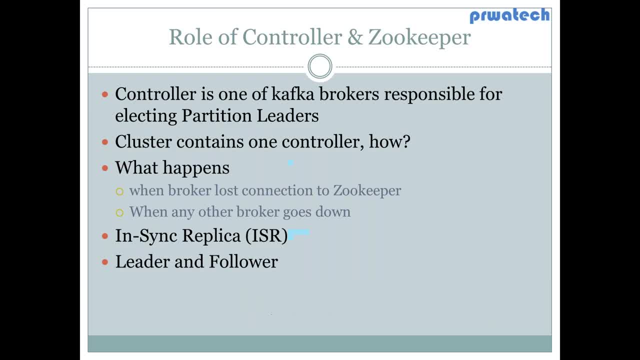 your parallelism depends on the number of partitions. okay, we go to the next slide. okay, so now we will this. we will little bit more, uh, deep dive into the kafka side. we discussed about publisher, who discussed about consumer, but i little bit skipped this kafka part. now we will go. 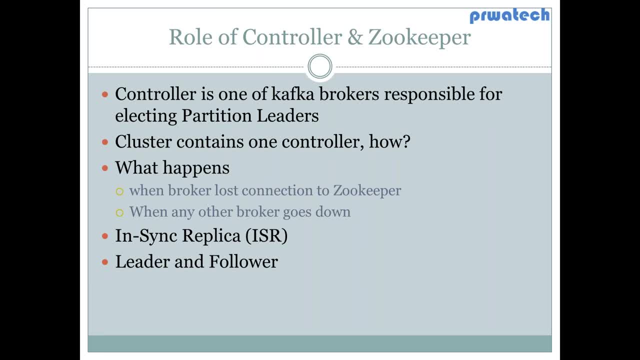 into, we'll deep dive into this kafka, uh, this kafka broker, like how, uh, how your data is being, how your message is being handled, or how this high availability and uh, communication things, how it is maintained, okay so, okay, so, control, uh. there are three, uh, there are three types of broker. 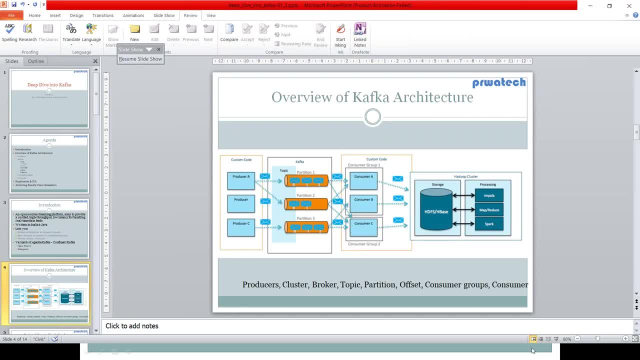 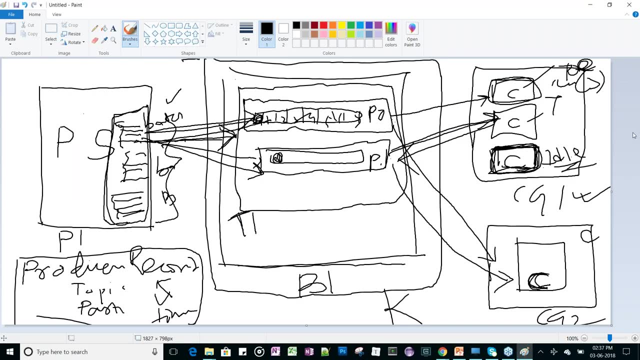 let's, let's have another picture, uh, and little bit uh more complex. hope you understand so far. any questions so far? uh, okay, can i get notes after this question? yeah, i will get ppt or give some notes. don't we get into duplicate data in consumer end? okay so? 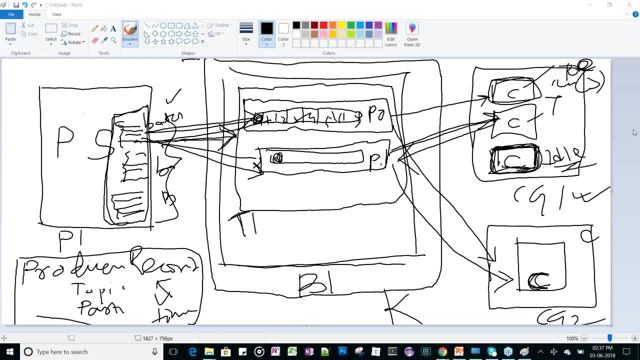 for that we have one, exactly one semantics. we will see in that, uh slide, how we were achieving, uh, how d duplication of message. okay, uh, for notes. uh, you have to communicate with pr. what team, uh and uh, they will get back to you. okay, and can you please record this as an? yes, uh, this. 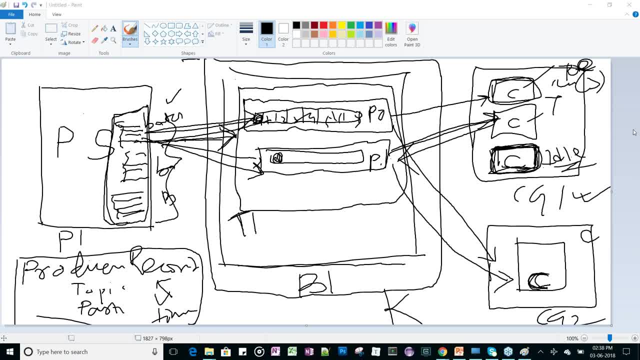 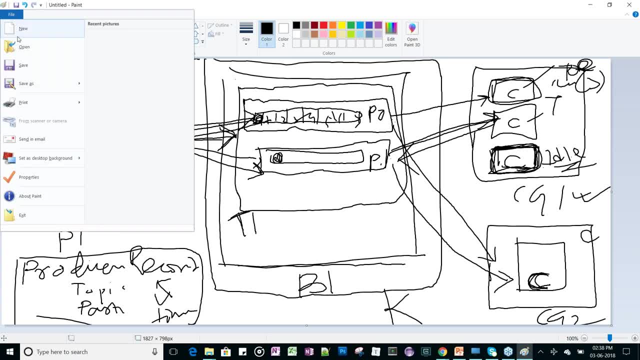 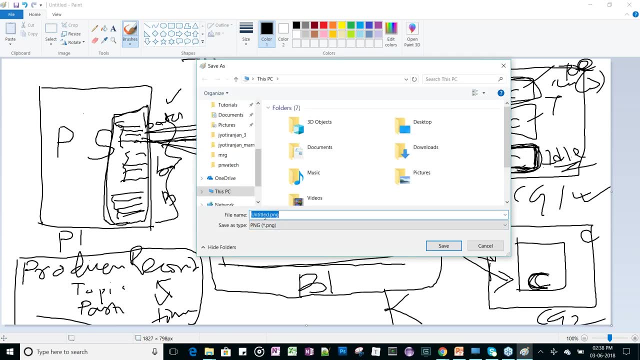 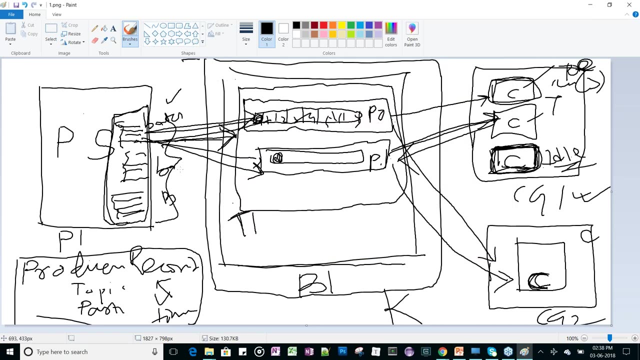 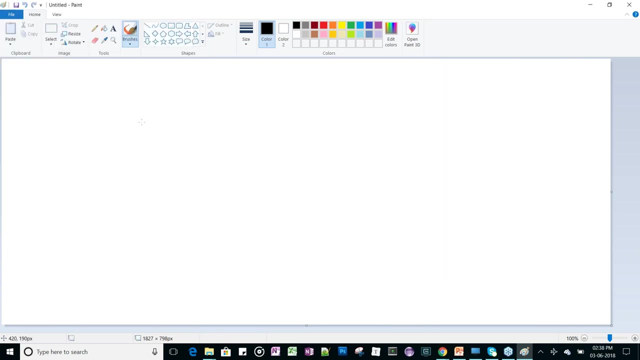 session is being recorded. okay, thank you. uh, so, moving forward, let me save, okay. so now let's have new, new board now inside your everything. now, now you are into the kafka, okay, kafka broker. so, uh, let's increase the complexity. it's not just one broker, three, two partition or three partition. 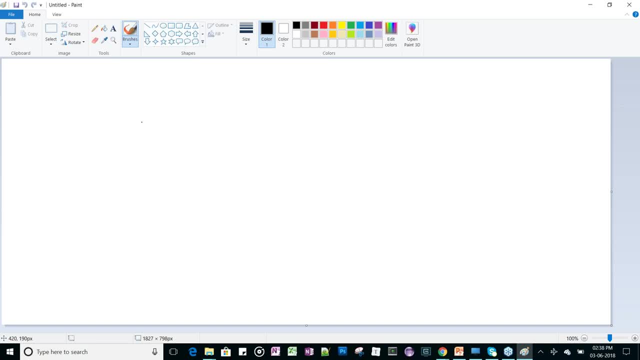 it's not so. there will be multiple broker in because you are dealing with a cluster. okay, so for example, uh, let's have this big kafka cluster and inside that we, uh, we have three broker. so this is one broker, this is another broker, this is another. okay, sorry for background. 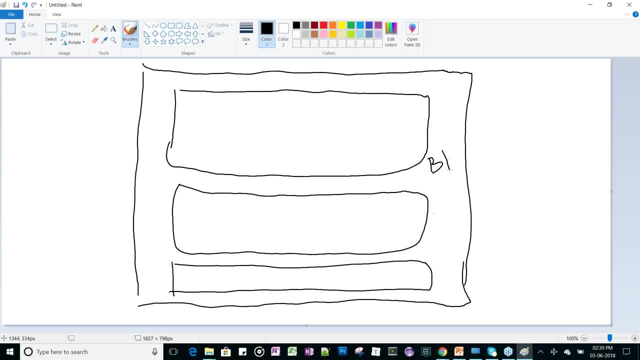 just, it's okay, so there are three broker. uh, okay, so this is a cluster now inside. uh, we have three broker. so there are two concepts: one is your uh partitions and then there is another concept called a replication factor. one is partition, another is the replication factor. okay, 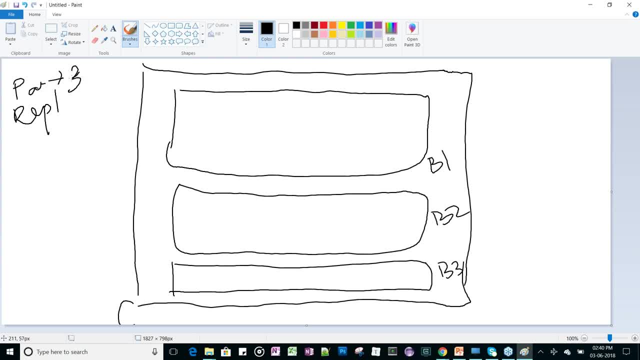 antriction: uh, so partition, for example. uh, three or two, let's, the partition has two replication, factory factor is three. you cannot have more replicas factor than your broker number. okay, so as we have in sdfs concept also replications, so two partitions and your topic has this: 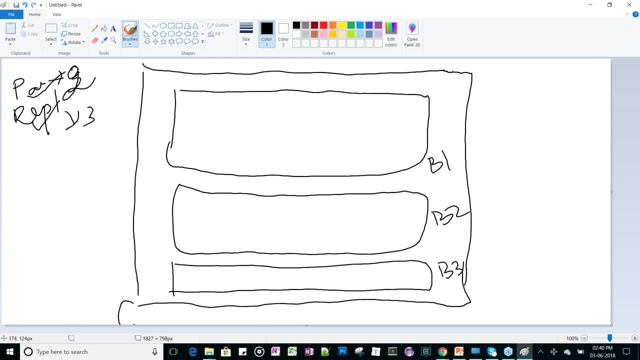 and the replication is actually this. partition or replication is actually on the con, on the context of topic. each topic can have different partition and different replication. so while you are creating a topic, you have to mention, uh, like that there is a topic, create a such command in that you. 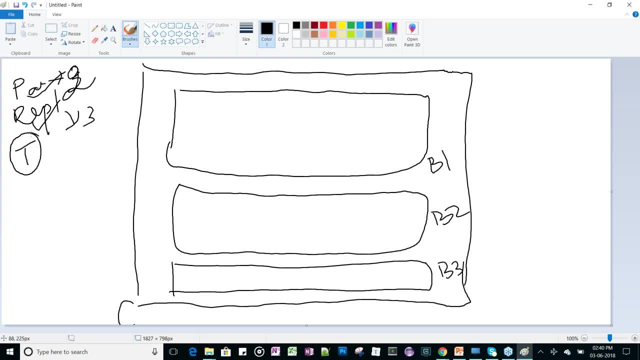 have need to pass some parameters and in that parameter you can have to. you have to pass partition and replication, okay, so going you will have in internet. also you can get uh in set up. it's very available, okay. or you can ask me later i will send you everything thing, is that okay? so 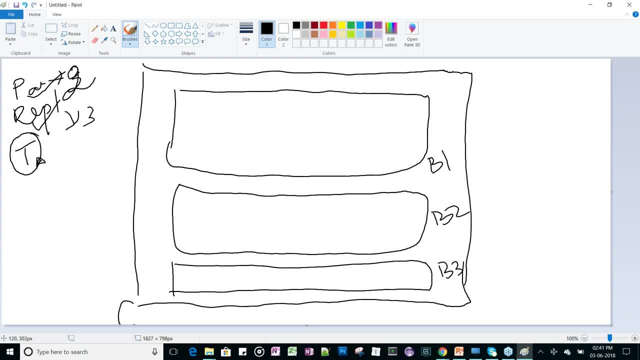 each topic. so we'll have a topic a and we have partition, two partition and replication. that means two partition, means that, uh, each broker will have two partitions, okay, so this is one partition and this is another partition and the replication is factor is three. that means these partitions like p a and pb. so this 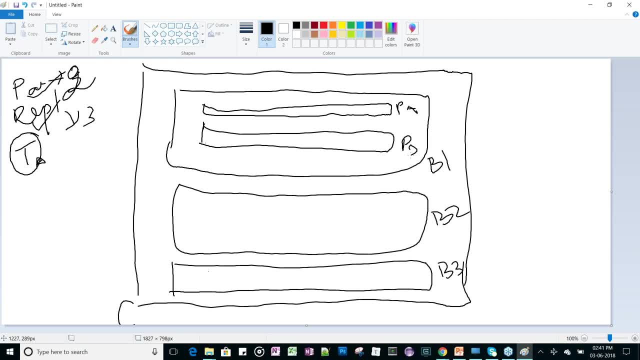 pa will have three replications, okay, uh. so that that means i i need to have at least three broker, at least if you can afford a four broker, but uh, the only, it will be replicated three. so this is one copy, okay, and another copy. is this one and another copy is this one, okay. so, pa, this is uh. 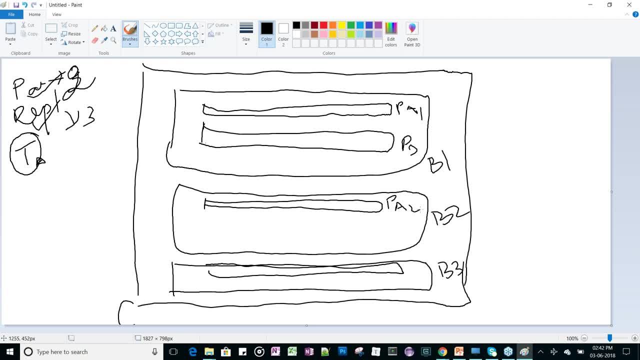 pa. for example, pa1, this is pa2 and this is ph. similarly, pb also will have another uh replication, so this is called pb2 and there will be another replication. okay, now, uh, uh. okay, so this is how your uh replication, your topic, is actually distributed. okay, 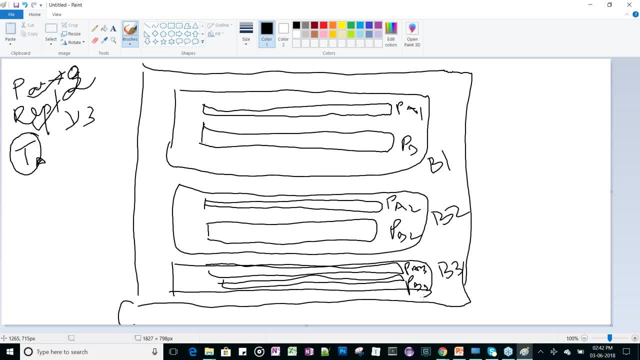 so now for one partition, for one partition, uh, there will be one leader broker and another two will be your follower. okay, so there is a concept called leader, follower, leader and another is followers. these are brokers, these are brokers. so so which will be the leader broker? for example, this for pa: this is your leader broker. 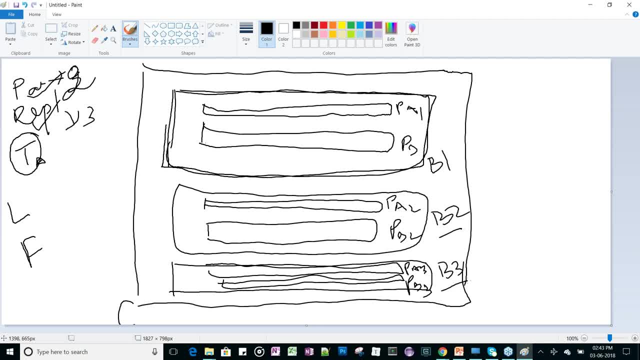 and p, b2 and b3. so for pa1, your leader is b1 and your follower is b2 and b3. for pb1, for example, your leader, your leader is b2, okay, let's say for lead. one for second partition, okay, uh. and for uh and your follower becomes b1 and b3. so one broker will be your leader. 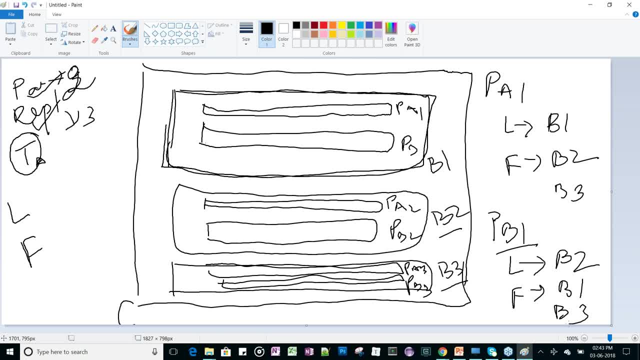 and another will be your follower. so when producer- okay, producer- will send the data and send the message to kafka broker, it will send the message to the leader, that message being will be handled by the leader broker, not the follower. the same partition. it is the same partition because we are replicating. 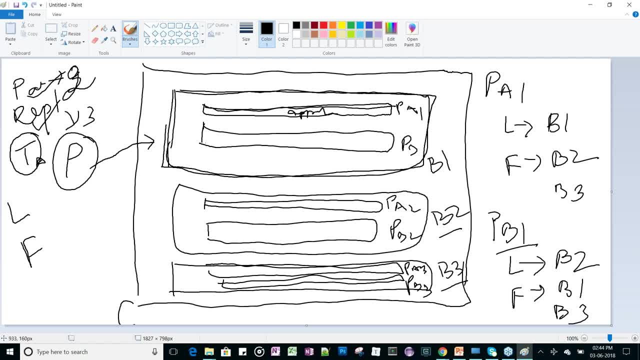 so if there is an apple here, this apple will be replicated to d here and also here. so the producer, producer. only send the message to the broke, to the leader broker, not other other ones. okay, not the follower. so far, Apple. okay, so it is going to the partition. one, like Apple, has some key, for example, a, a for Apple, a. 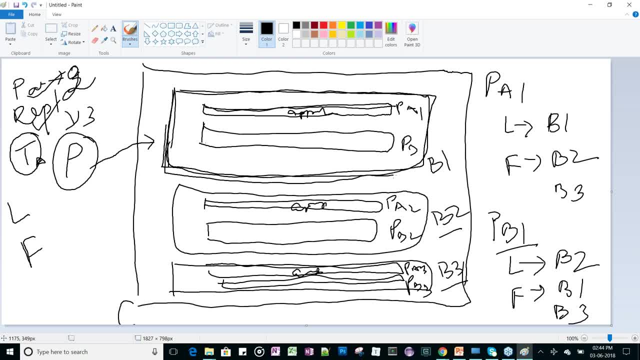 is the key and for party some partition logic, it is going to the partition PA 1, partition a: 1. okay, so it is going to that b1 leader, because for partition one leader who is the leader be one, so it will go to the leader leader. this 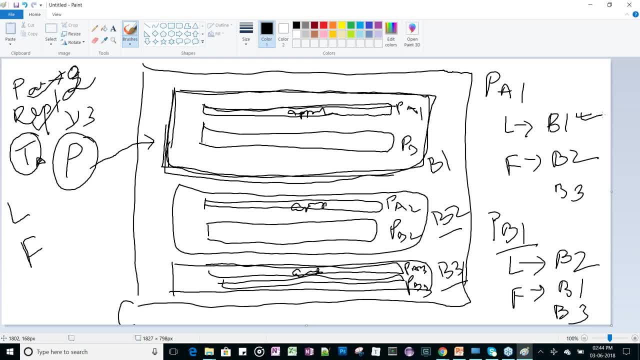 message will be handled by the leader only now, for there is another. for example, BB for a ball. another message before ball that producer is sending for the key B. it should go to the P B, P B partition, second partition, but the second party leader for the second. 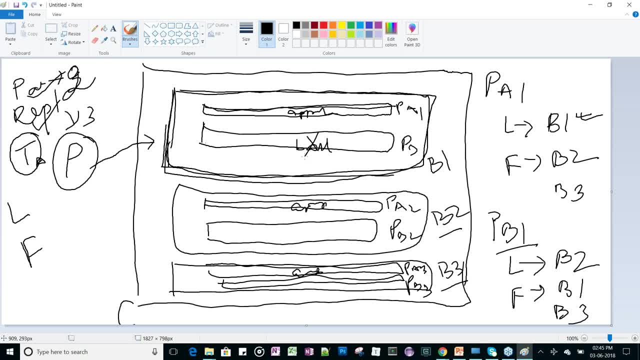 partition is going to the P B, P B partition, second partition. but the second partition is B 2, so ball will not go to here. all will go to after that. this, when, when you this, because for the leader, leader broker for the B, but this partition is B 2, so it will go to the leader for that partition, so B 2 now. 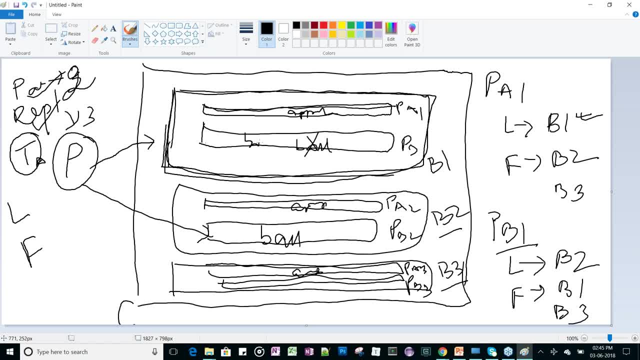 after that it will be replicated. this ball will be replicated to here and this one will be related to other follower broker. similarly for Apple also, this Apple B one will get the data and Apple will be replicated into P a second to a follower broker and then part of it. okay. 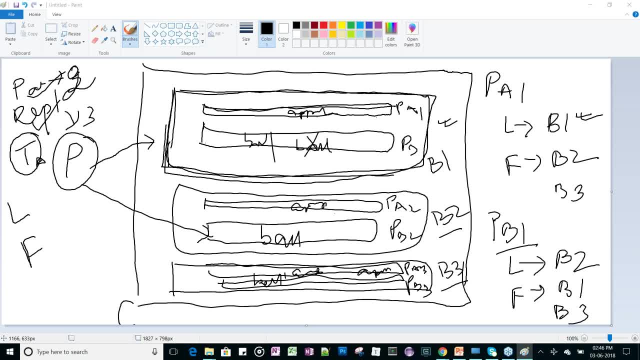 so one is leader. so one is leader and another is follower. now thing is that who we will control this leader and follower. that means when who will select a broker, who will select a broker? and who will control this leader and follower. that means when who will select a broker, who will 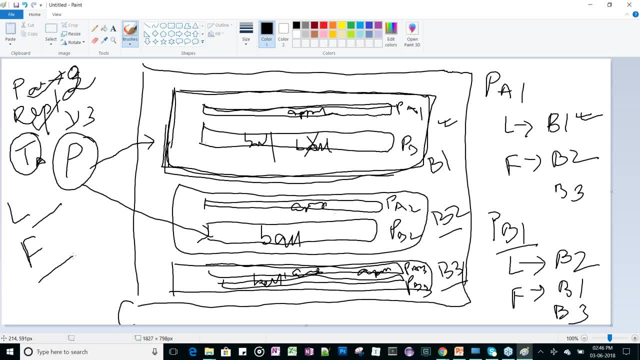 select a broker as a leader- broker for a partition- and who will select a broker as a follower, so that role is being managed by controller. so controller is also another broker of Kafka. well, let's, it's not a separate thing. for example, you can imagine that this B one can be a controller. this broker can be a. 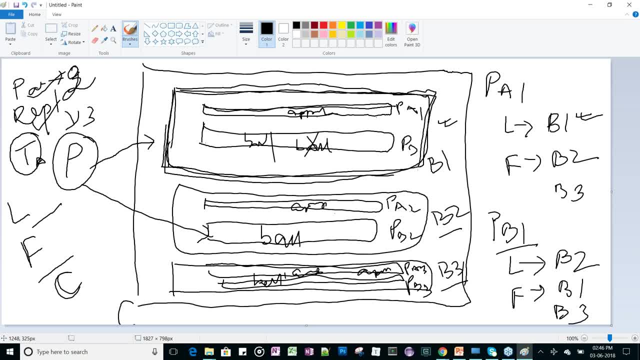 controller broker. okay, controller broker, who is who will? who will decide which will be the leader? okay, which will be a leader for a partition and who will be the leader for another partition, like lead, who will be the leader and who will be the follower? that is controlled by your controller, okay, so when? 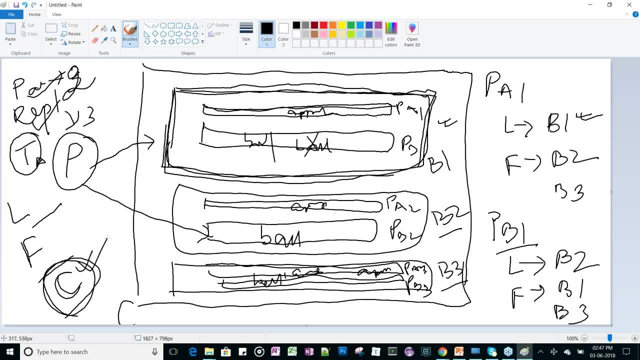 you when this controller will play, will have its role when you will start your Kafka broker, right, so when we will start your Kafka broker, at that time you are, you are starting your Kafka cluster. so you are starting your Kafka cluster. inside that you have three server dot properties file for each server dot. 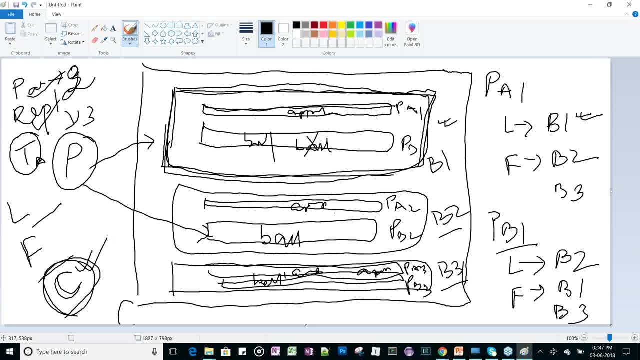 property file corresponds to a broker in the configuration. so you have three server dot properties file corresponds to the three broker. now, when it will start at that time, one broker among them will be the controller. okay, one broker will be the controller and until now there is no leader, follower only. 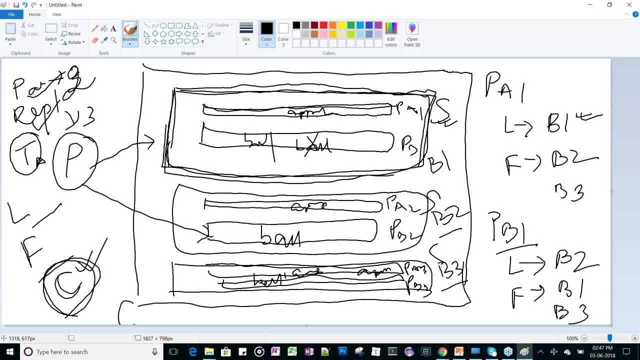 controller is being decided now, when we will create the topic. at that time you will decide how many partitions you want, how many replication you want. okay, so a many partition you want. accordingly, it will decide. okay, so there will be two partition will be created for that topic. so okay, for these two partition. who will be the leader? 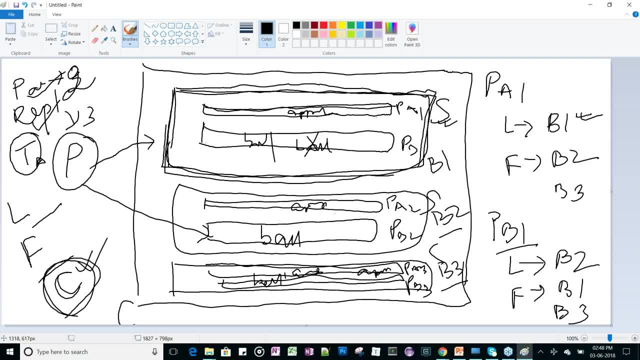 who will be the follower. that will manage by your. uh, okay, so come into picture. then, when topic will be created, at that time leader and follower will come into the picture. okay, understand, so far, any doubt? uh, okay, let's go to the slide. okay, a bit more, so hope you are seeing some new things. 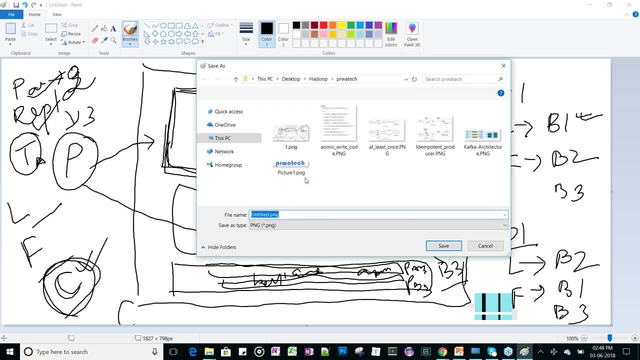 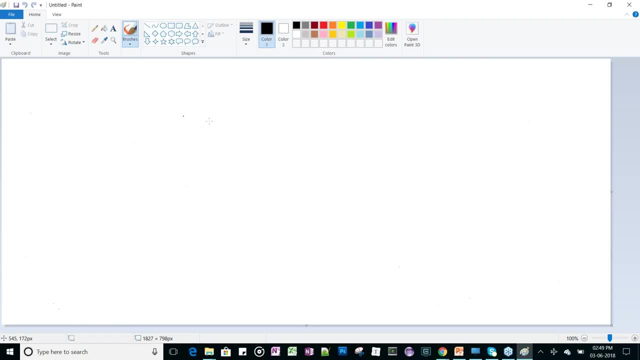 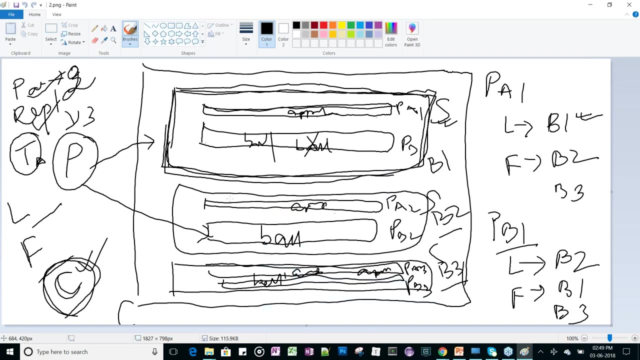 because there is so many uh articles on kafka. it's a bit of beginner and intermediate level. so now uh thing is that. now let's see, okay. okay, here one more point is called in sync replicas, isr. what happens is that uh, apple went to the partition pa1. okay, now this message will be replicated to pa2 and pa3. 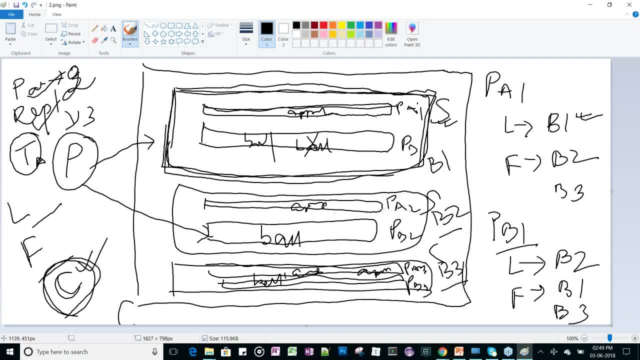 so each follower follower always uh follow the broker, right, so uh follow the leader. so this follower always keep fetching, keep fetching the data fetch request, keep sending your fetch request for to the broker, to the leader broker. okay, so this, can this follower broker keep sending their uh fetch request to the uh leader broker? now, if, when, uh? 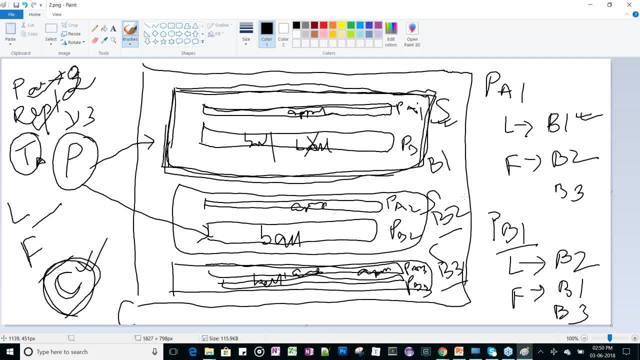 when they will get the apple, all these, all these broker will get the data. all this follower. when this, all these follower, uh broker will get the data- apple data, uh, then it will call uh, then it will be called as in sync replica. so these replicas are in sync, are in sync with, in sync with leader. 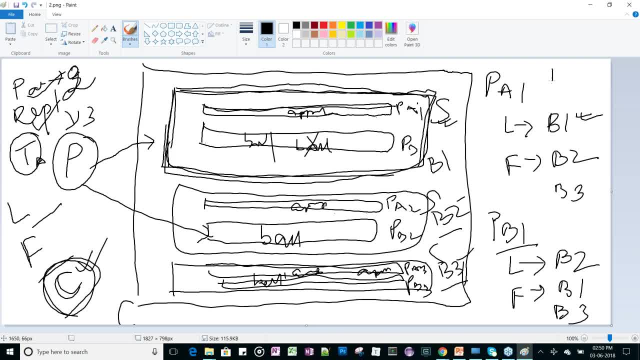 okay, so, uh, so there will be another index, isr in sync replicas. and why it is important? because this, uh in sync replicas, uh confirms your consistency of your record. if one broker will goes down, uh, then the, for example, this leader goes, goes down, then only among these in sync replicas. in sync replicas, uh, only among those broker will be, uh, your leader for. 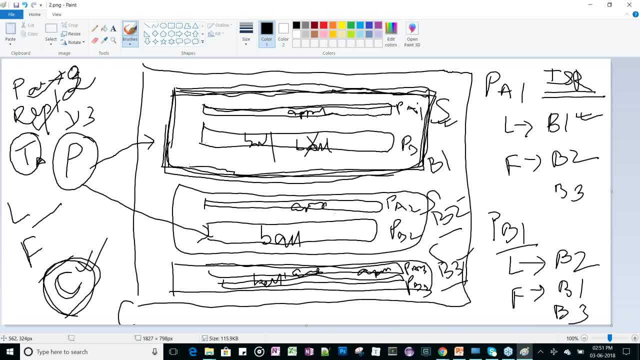 example, let's say two, the apple is uh replicated to b2 but not b3 somehow. okay, maybe there will be network condition. uh, maybe there is some memory issue. so this b3- uh, your data, apple data- is not- is not uh present in b3 broker so far. so, uh, it's not uh, b3 is no. 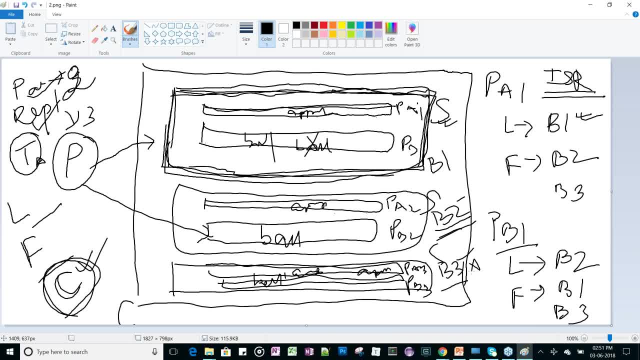 not in in sync, in in with in sync with the leader broker. so, uh, when this b1 will go will go down. at that time, uh, the controller will choose right who will be our uh next leader. so, at that time, only from this ion in sync replicas, uh, it will choose uh your next leader, not me. 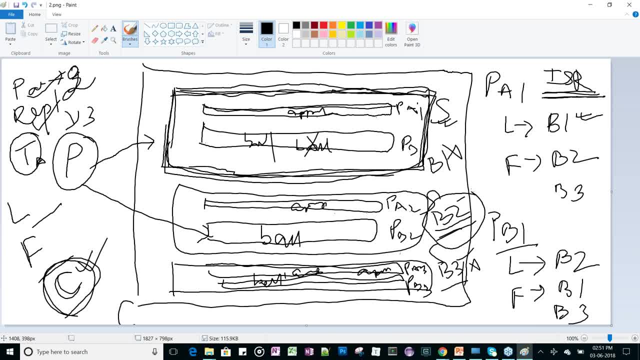 and your uh data is also, kind of it, a bit unsafe because your data is not in, not in sync. your consumer also consumer also- will be able to uh consume the data. which, which data are actually in sync. okay, uh, so there is two concept: uh read committed and read uncommitted. that i will explain in exactly one semantic. 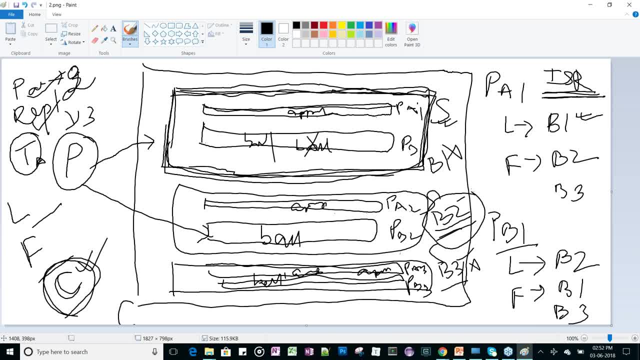 so thing is that consumer reads data from in sync, replicas only in sync. which? those data which are in sync? that means those data which are present in all the all the broker, in the sense of how many replication factor? you have mentioned that number broker? uh, those that are in sync, and those data only can be read by the consumer. now there is some. configuration tweaks. also you can min. you can tell uh the kafka broker that okay, though replication factor is three, but consider two as uh in sync replicas, like if your data is present in two broker, then also consider it as in sync at that time that data also uh can be available for consumer even if there is another broker. 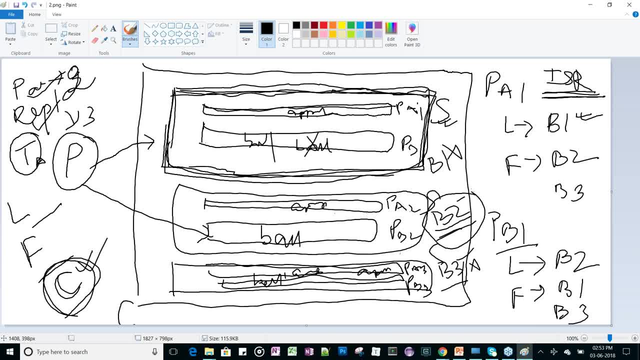 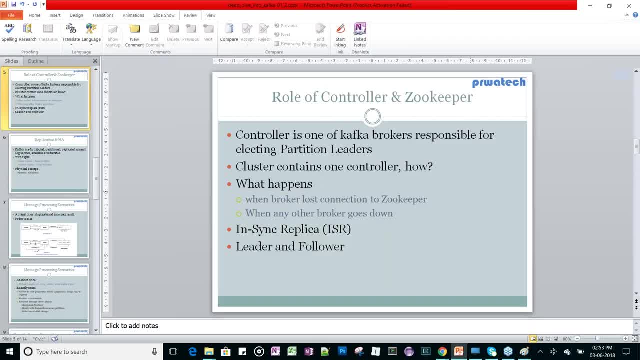 which is, uh, which doesn't have that. that configuration is also there. i'm just telling from the concept view that, okay, there is some provision you can check. okay, because in this one hour the so many concepts to complete, it's a little bit difficult, uh. so i'm just giving a conceptual right and i'm just telling what are the provisions? are there? so? 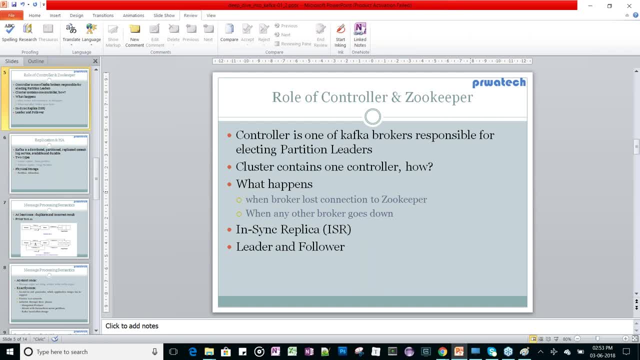 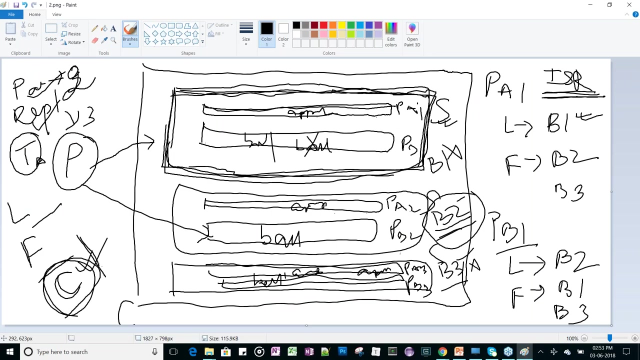 you can read documentation. there are a few blogs. cloudera blog is also there and you can get some ideas. okay, so controller is one of kafka broker responsible for electing partition leaders. okay, we discussed cluster contains one controller. this cluster contains one controller half. let's discuss how. so this controller only leader. leader is one and uh, follower can be many. 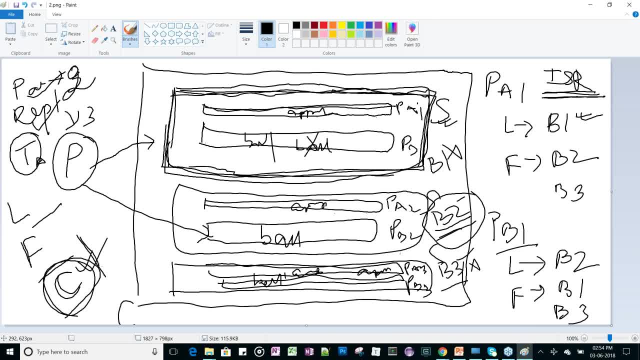 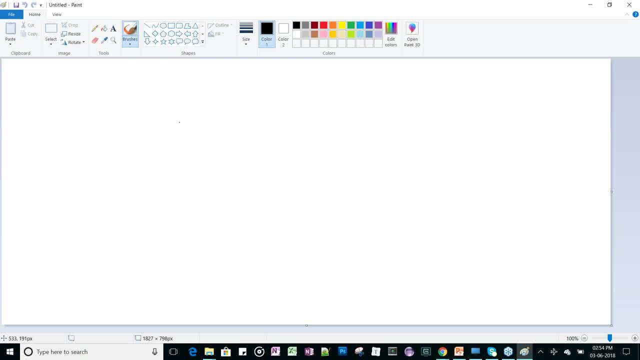 uh, but so thing is that this cluster, how this cluster thing, are really managed only one cluster, so you from two keeper perspective. okay, so now, when your kafka bro kafka cluster starts, at that time, uh, at that time you have mentioned three brokers, because you have three server properties. 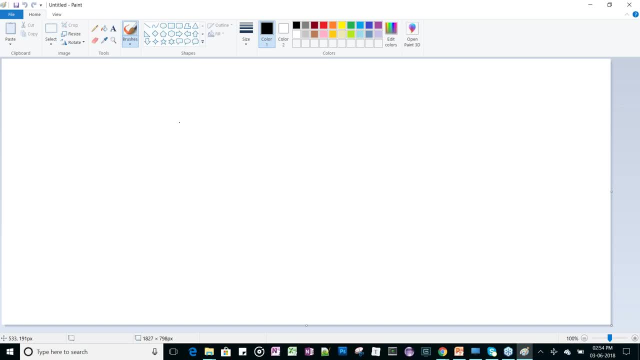 you can have one server properties or one broker in that case. but we are discussing leader, follower, controller. that's why i'm just making three broker scenarios. so uh, okay, that's one time okay. so uh thing is that, uh, when you have, uh, your capital cluster starts, capital cluster starts, at that time three brokers. so for 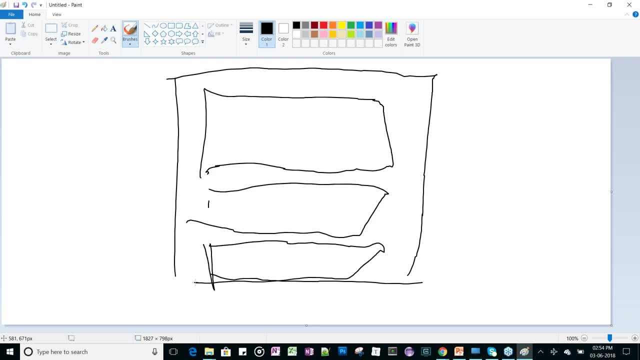 one broker, there are three broker. for one broker, there will be one, uh, in the zookeeper- this is your- in the zookeeper, for there will be one slash con, one id slash control. so, uh, the which one one will be chosen from this broker, whichever first created, and it will create, a. 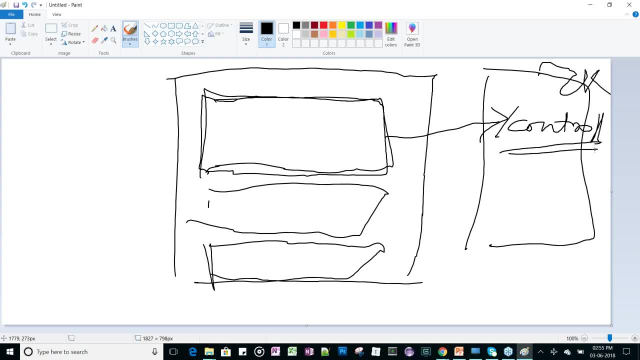 directory in the zookeeper called control. okay, so that will be your uh controller, another one we may try to connect and try to create control, but it won't be able to because it will throw that. okay, controller already exists, so there will. there will be further controller will not be able to make. 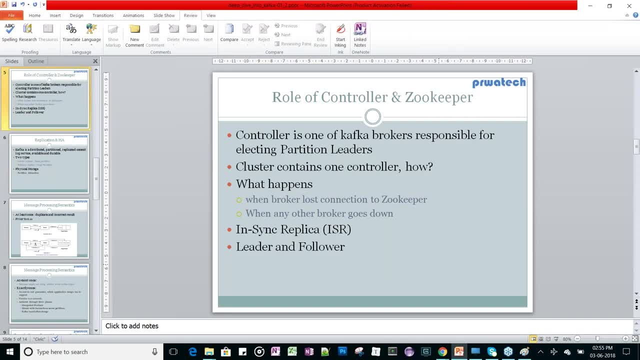 so there will be only one controller. so what happens when broker lost connection to zookeeper? so we discussed, like broker when broker will in the broker. in the sense i am telling leader broker, okay, when leader broker will lose the connection to zookeeper, at that time another. 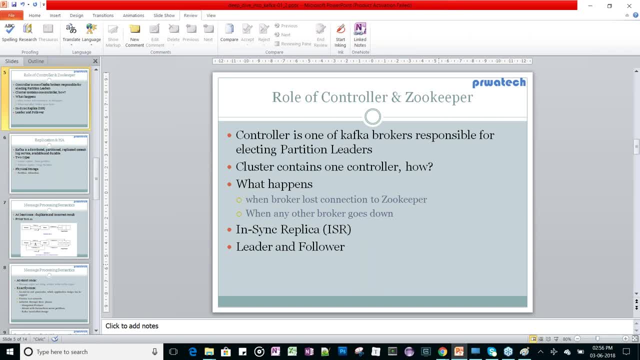 one i discussed already, so another uh uh, which is in sync, with which another uh broker, which is in sync, will be the leader, will be the leader and there will be corresponding entry in the zookeeper. okay, uh, so that will be managed by controller. now, when any other broker down at that time, so any other broker, like follower broker, goes. 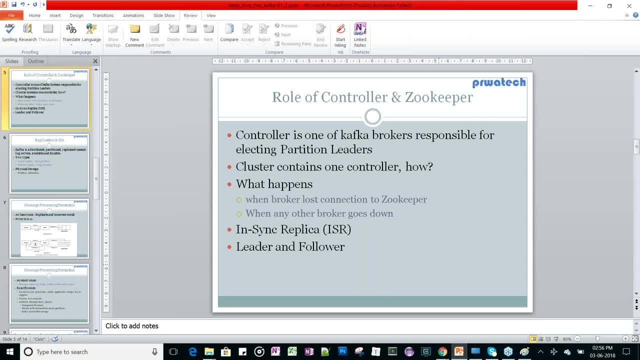 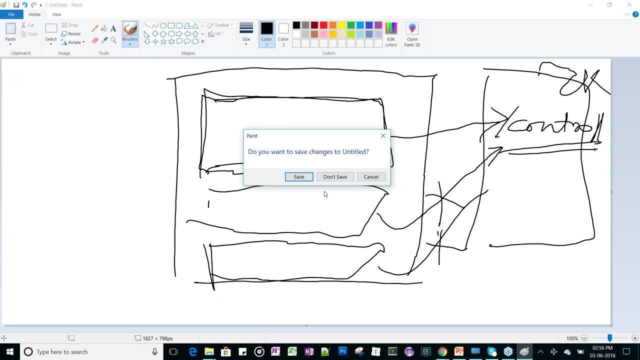 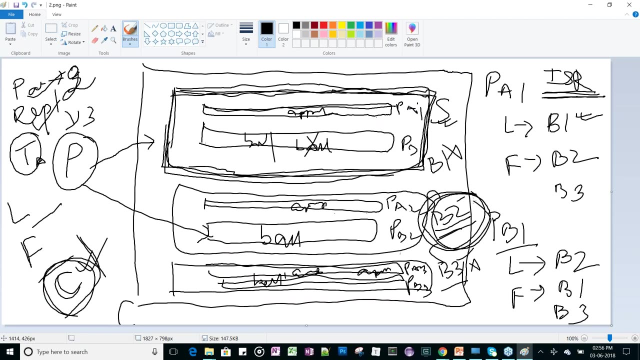 down. another scenario: when another broker goes down. so uh, for example, let's go to this image: okay, so, for example, this v2, b2 goes down, but b2 is the leader for this partition pb. okay, so, uh, the controller responsibility is that. so another broker for b3, b4, comes into picture. 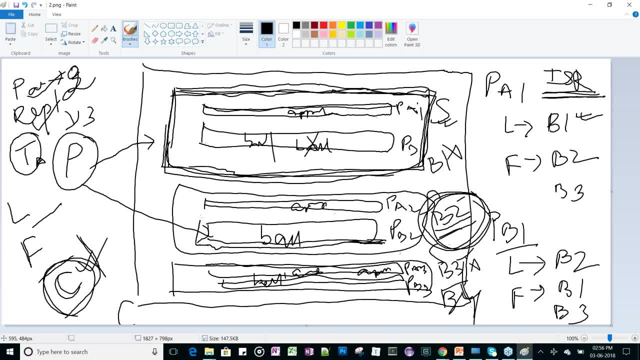 okay, b4 comes into picture first. it will just, uh, handle this leader partition. the partition, i think, is that uh, for the partition which is for which it is the leader. so b2 is the leader for b partition. so that partition is moved to b4. it is being handled fast or in, b4 is taking time then. 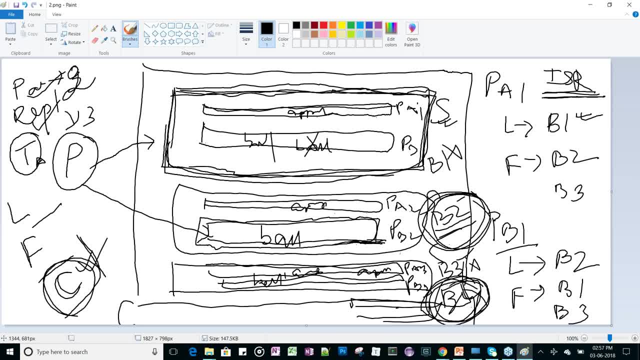 this, uh, if b4 is taking time to get up, so at least pb will be managed by other other, any other partition or any other? okay, uh, after that. okay, so this follower thing will be managed, but for which the leader, uh, for which the partition? for which partition the leader, uh, the broker was the leader that partition. 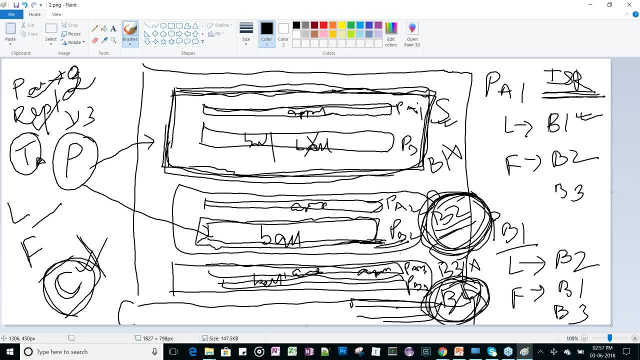 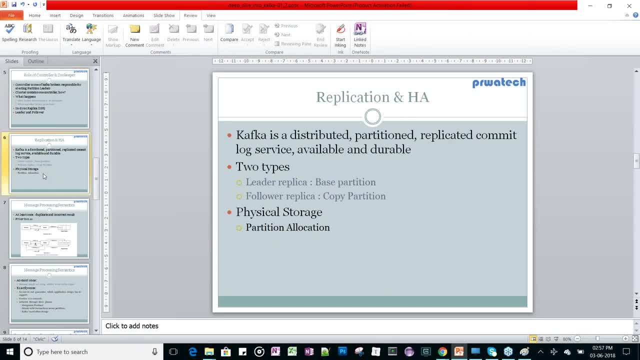 is being handled fast in sync replicas. we discussed and leader and follower also. we discussed the next line, because we have time constraints, replication and ha. so kafka is a distributed partition, replicated, commit log service, available and durable. so i discussed, like how it is partitioned, your data is partitioned and 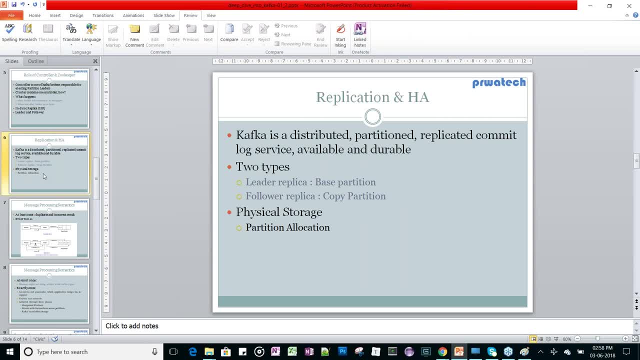 replicated. commit log services means there are multiple partitions, are there? uh, there are two types. i also discussed leader replica and follower replica. leader replica contains the like was the best partition, your base partition. that's your leader and the follower will request the fetch request. it will send face request and it will have. so that is a copy. partition: follower replica. 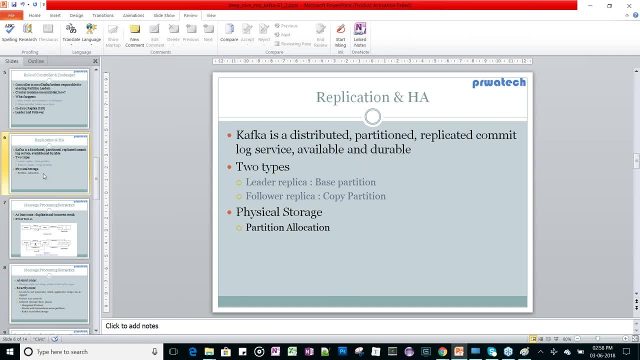 physical storage: partition allocation. physical storage- also i mentioned in one of your questions- is that it will go to tmp slash, tmp slash, kafka and locks in that directory. there will be a, there will be a direct in that directory. there will be a directory for each topic: partition. 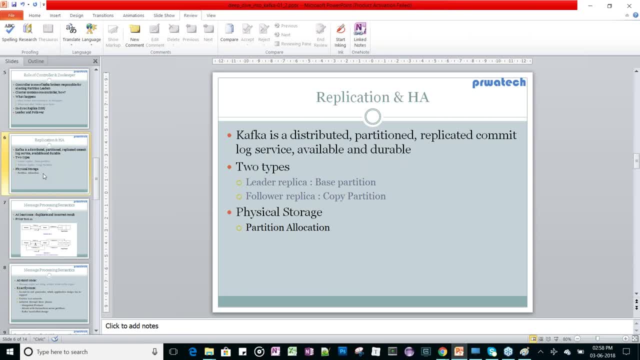 so topic 0, partition 0, there will be a directory inside that there will be two files: one is index, another is for your storage, your actual data. so that is mentioned by log dot dir in configuration, in server dot properties file. okay, so now, uh, we'll. 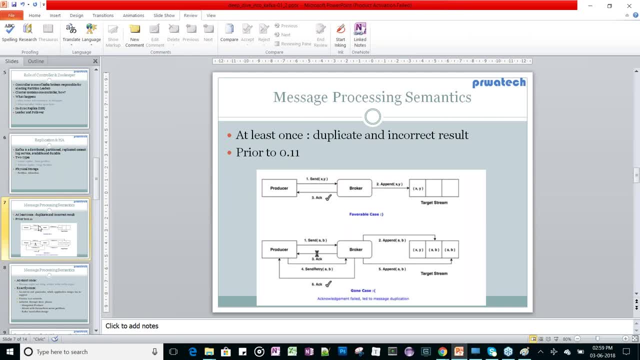 go into the message delivery semantics, like how your message is being delivered, like at least once, at most once. actually there are three kinds of message delivery semantics. one is at least once, at most once and exactly once. okay, so in at least once. at least once means let's say, uh, and it is. 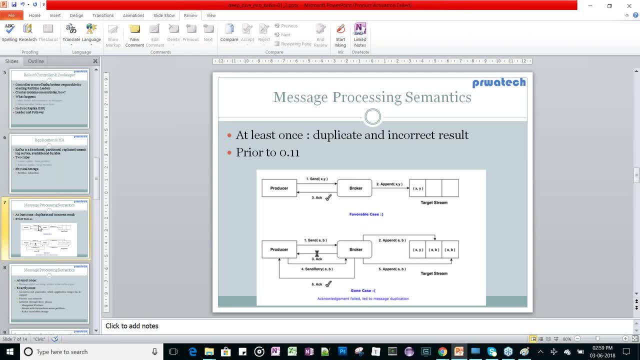 it was before 0.11. now the kafka version is like one dot, something is there, so, uh, but prior to 0.11, uh, it was only at least, it was satisfying, only at least once. so there will be, there will be duplicator of records and there can be incorrect results prior to 0.1. okay, so what? what was? 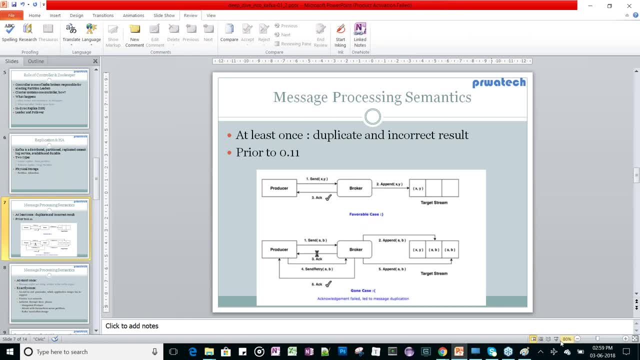 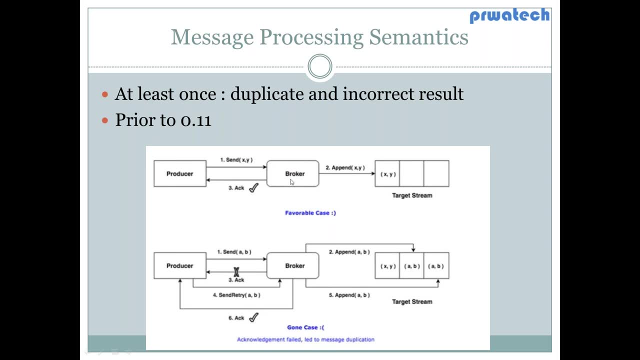 happening. what's the problem there? so here you see: okay, producer, producer is sending data- xy, for example xy- to the broker. now this xy is being uh, is being uh transferred to the your consumer, like xy is okay, consumed. now this broker is sending an acknowledgement to the producer. 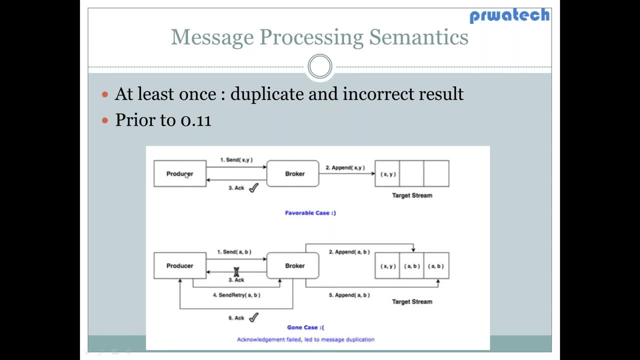 so there can be like the in the publisher. also, you can have three types of acknowledgement configuration: x, s, e, k, s, x all or x 0 or x 1 x 0 means there is no need to, no need of acknowledgement from the kafka to x. equal to one means one your when your message. 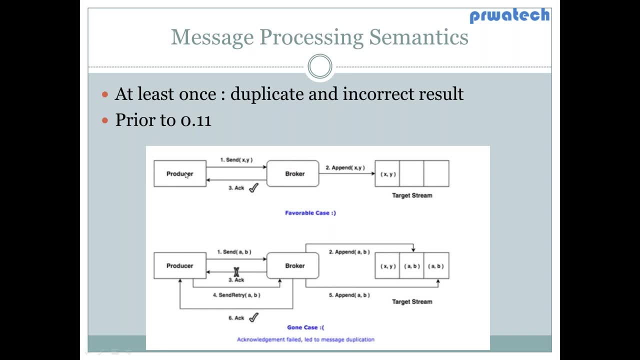 when producer will send the message to the kafka broker and your leader leader broker gets the data and it sends acknowledgement, that is, it will check for only leader gets or not. so that is a c case, x equal to one. now the third one is x equal to all. that means your uh, all your uh. 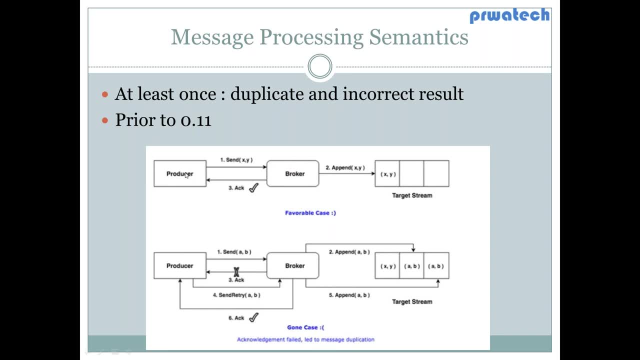 followers also will get the data. after that, only your acknowledgement will be sent to the producer, so producer will wait till the time. uh, all your leader and follower will get the data. so that will be a little bit less. so x equal to one is pretty good, okay. so here we are considering. 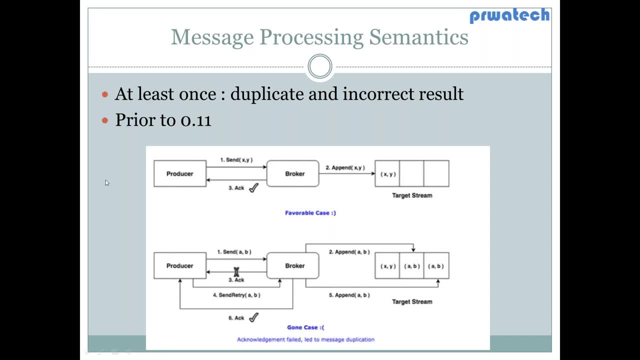 x equal to one. so broker is broker is sending acknowledgement. now this is a good condition, okay. producer is sending some message. that message is being consumed and producer is sending the consumer uh to. broker is sending that to the producer. it's a good one. now there is a real tension. what is the bad one? so what will happen? that producer? 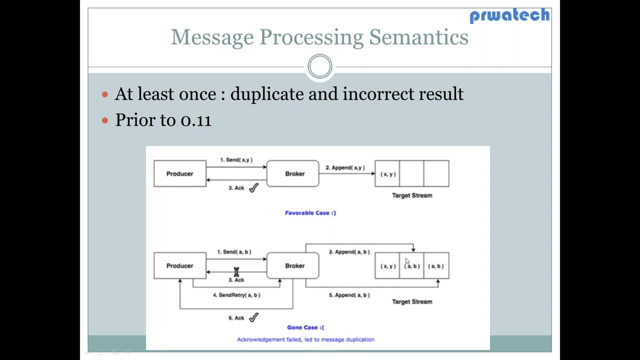 is sending message to the broker. broker is sending them. okay, that message is being pulled by the one consumer. so xy y, x, y is all. uh was always, was there already, so now a b came. so a b came. okay, now broker is sending acknowledgement. but something bad, there is some network or something. 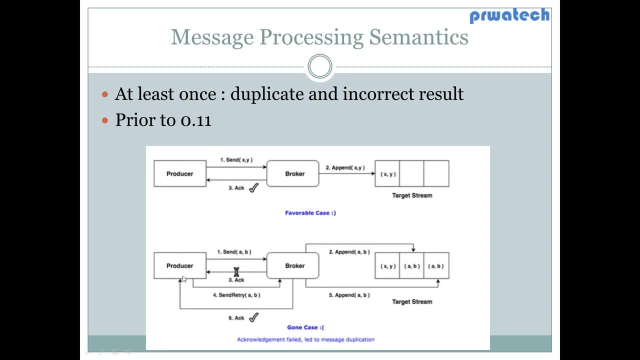 happened, it's, it didn't. uh, it was not able to. so producer now doesn't know that message actually get persisted, consumed, lost, what happened to that? so again it will send. retry the message to again. it will try to send the message to the broker now. broker will again process the data. 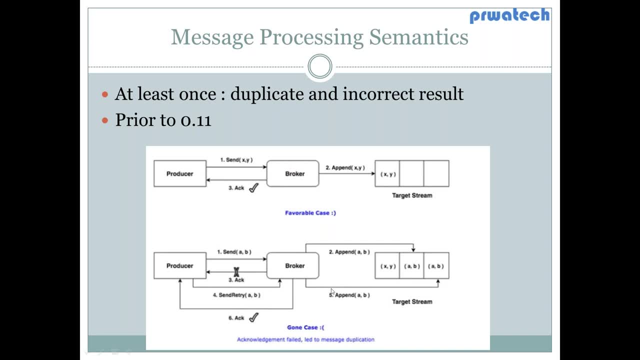 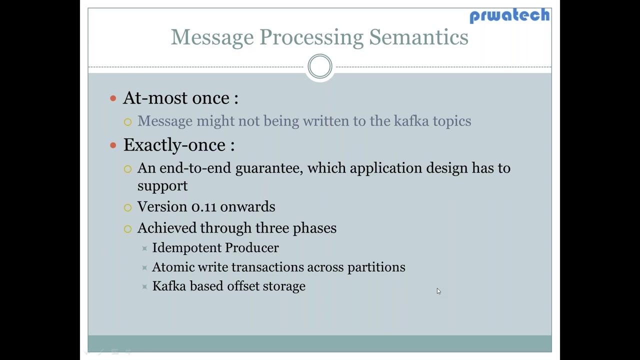 so a, b will come second. so here, uh, there will be duplicate and there will be acknowledgement. that's right, so okay. so now. the problem here is that there will be duplication of data here. you can see a, b. okay now, uh, the second one is that at most once, okay, at most one, that means message. 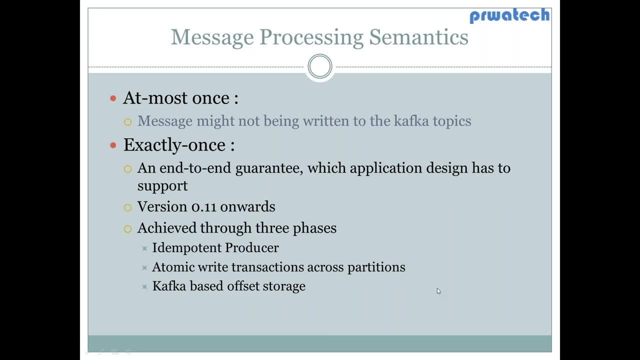 message may be. message can be lost at most once, but it will just send the message and that's it. when the producer will send the message, this data is being persisted or received it, or the consumer received it. nothing, no need to uh bother. in that case, your message. 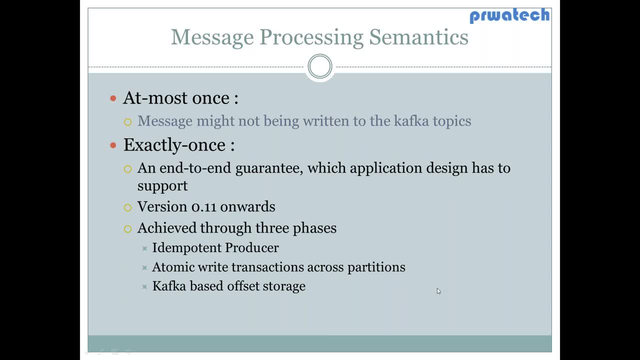 can be lost. it's not advisable to have at most ones. so at least once at least was there before zero. so now the challenge is that they are to have this exactly one semantics: how we can have end-to-end guarantee that your message will be: um persist, consumed only once, persist only once. 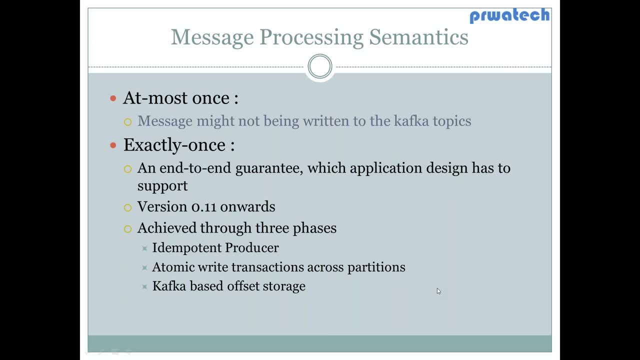 by kafka. so that's a challenge in any distributed messaging system. okay, so after 0.11 only, you can have this exactly once. you can achieve this exactly once, but let me tell you that it's a end-to-end thing. okay, so you have to uh your producer, your kafka, and 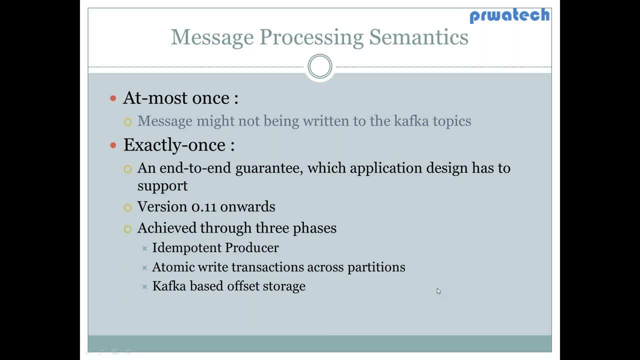 you're also a consumer have to follow some rules. some rules to uh, or to have such a design decision, uh, to have this exactly one semantics, but it will save you from deduplication. okay, though, there is some uh scenarios that where this exactly once will not happen, but most of the scenario it will be uh. 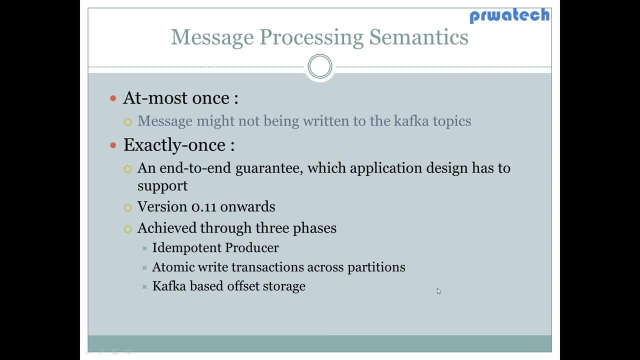 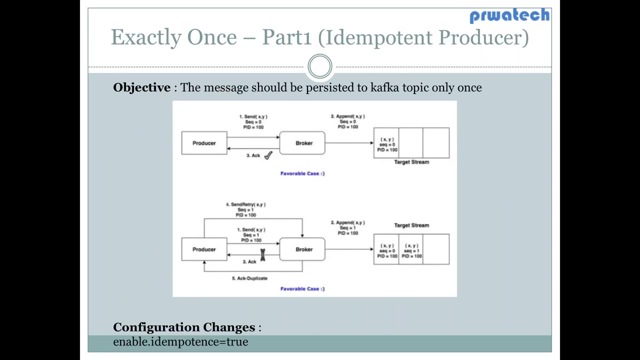 covered this exactly once will be there. so this exactly once uh scenario. uh is achieved by three phase. okay, one is idempotent, producer, atomic. then second one is atomic right transactions across partitions. another is kafka based rules. we will go one way, so exact, idempotent. 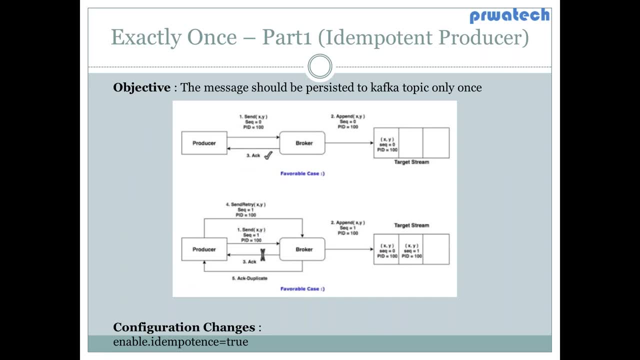 producer. what does that means? i don't put it. producing, okay, so this exactly is one. semantics is divided into three parts. okay, produce, so it's an end-to-end guarantee guarantee. so producer has to, uh, maintain some rule and then kafka, broker and then consume. so let's see from the producer. 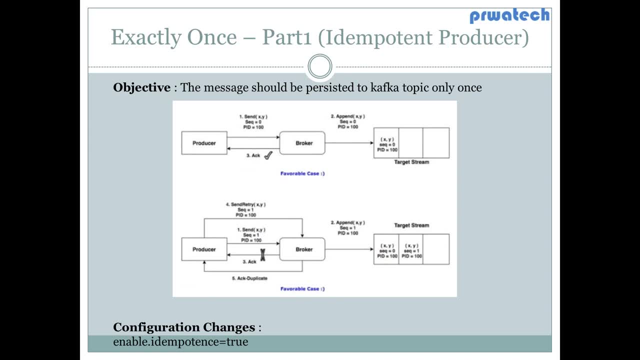 side. okay, producer to cup in this part, idempotent producer in this part. the objective is the message should be persisted. persisted to kafka topic only once. okay, how we can achieve that. so producer has uh here, producer has uh here. actually we have two id. when producer sends message to the broker, there 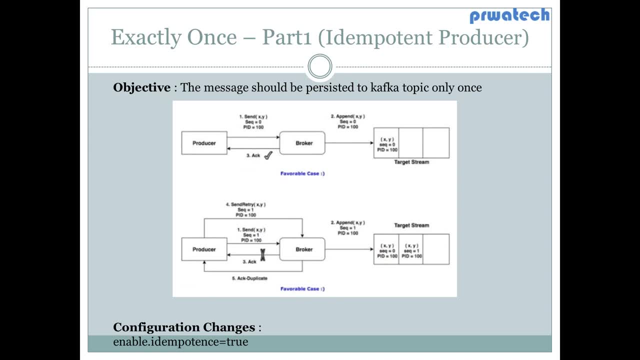 are two, two id involved. one is p id, that is producer id, and another is sequence number, that is for sequence number per message. okay, so let's say your sequence number is zero and your producer id is hundred. okay, producer id is hundred and sequence is zero, so it is being sent to the 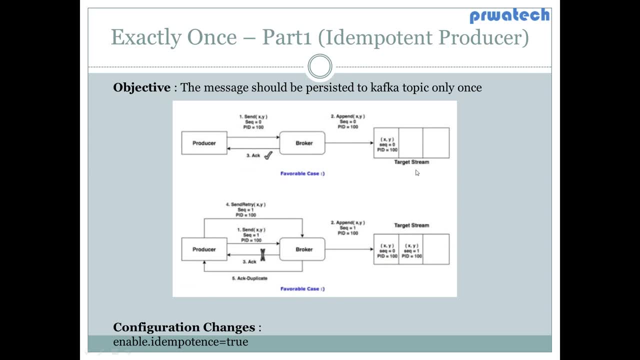 kafka broker. now kafka broker is sending to this: uh is consumed by this target stream sequence: europe. this is a good condition and it is sending the acknowledgement. okay, let's see the bad condition, the favor, the unfavorable case, so how it is handled there. so that was our challenge, right? 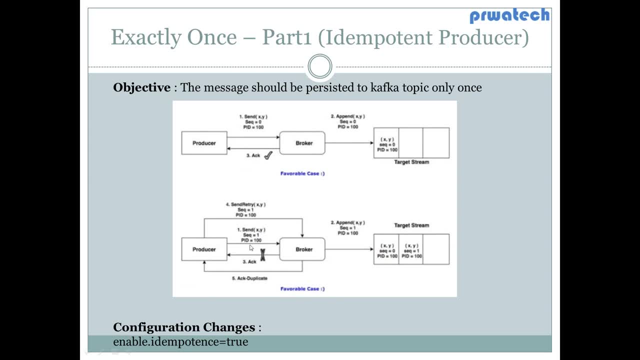 so producer is sending- producer is sending this x y message with sequence number one and, uh, your producer id is hundred. it went to the broker broker stores message, sequence one and process id: uh, producer id equal to 100. okay, now, while while acknowledgement, if something bad happened, that was our scenario, right? 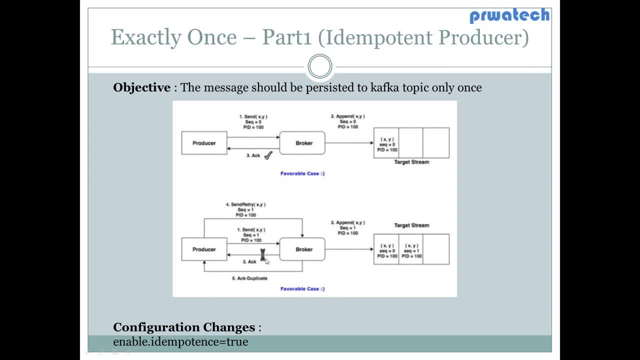 how we are, how we will handle now. that's the challenge. so there is some acknowledgement, there is some issue with this acknowledgement. so now producer, again, producer doesn't know- okay, his message, my message persisted or not? so again it starts sending, sending this sequence with sequence number one. again same message, sequence equal to one and its. 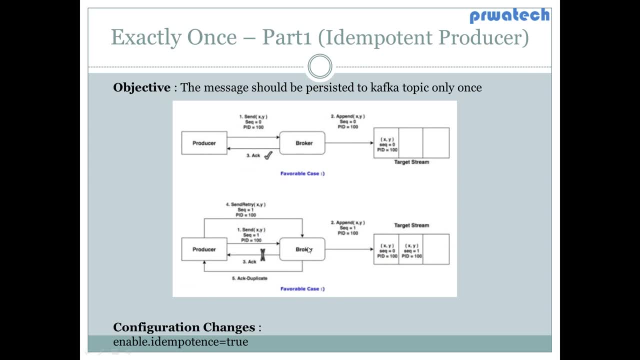 producer id is called hundred. now this broker, now the broker knows, broker knows, okay, with the same pid, the process id and for the same topic and partition id, because it's a uh, in kafka, 0.11 of wars it checks, that is, is it the same process id that i processed for the same topic or partition? 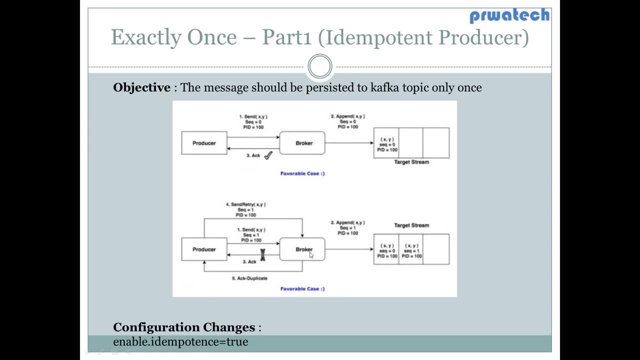 only one pid. correspond to uh, correspond to topic: each topic partition. okay, so now. okay, yes, already i processed it. this kafka broker knows, so it will not further process it and it will send acknowledgement duplicate as a response. okay, so the producer will get an. okay, my message is: 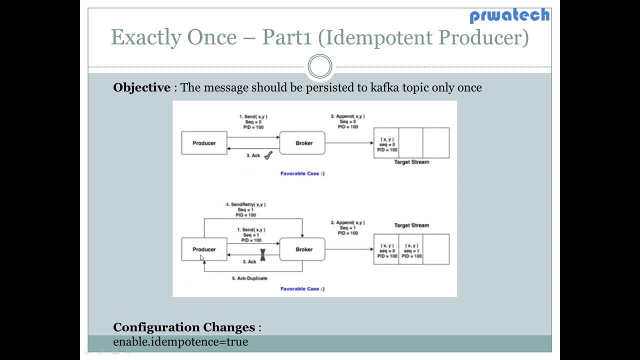 persisted. it doesn't need to work so to uh. this is how this one part producer took producer to kafka. that part is solved. we'll see the next consumer side also because it's an end-to-end guarantee. now, to enable this, just we need to have enable dot item contents equal to true in your kafka broker. 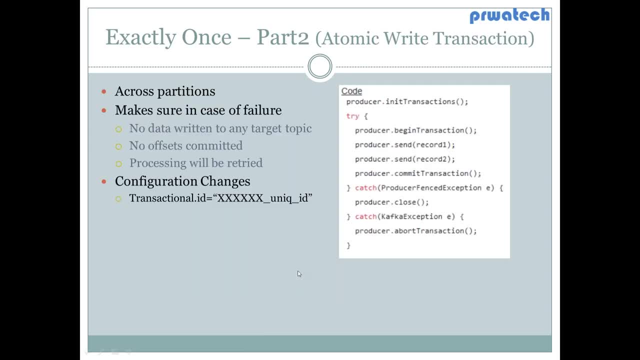 okay, the second part, then the second part. you need to think about your, uh, your kafka broker part. okay, so how, when, when this, uh, i said this is the only producer to one partition, so you have across partition, so producer is sending a message and that message will go to: 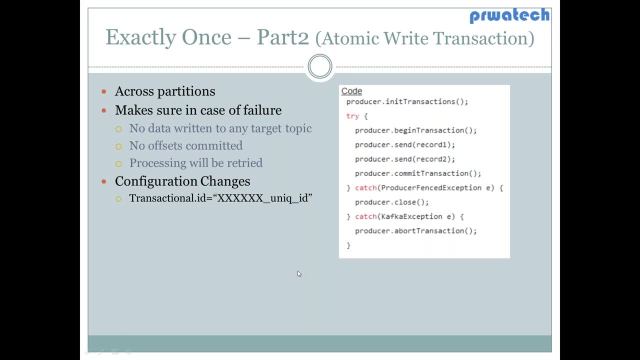 one partition. one message will go to one partition because of partition, partitioner logic. but that batch contains many, many messages, so those, all those message can go to different, different partitions. okay, so in one partition, uh, in one partition it message actually delivered, but in another partition message didn't deliver. for example, there is some network issue. 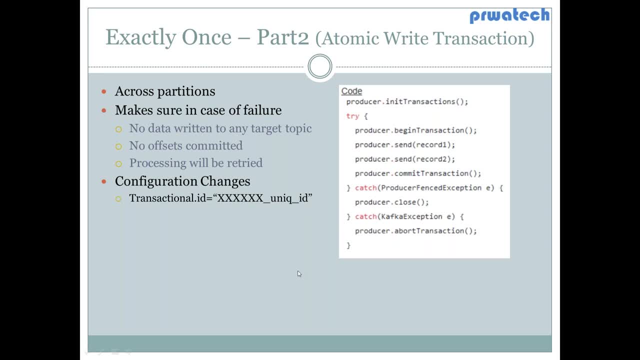 okay, so in that case there will be problem, right? uh, you, and next time when producer will send the kafka, broker will tell that. okay, i have already this process: id and partition id combination. i won't process your data acknowledgement. uh, it will send the duplicate acknowledgement, but your data is lost. uh, in the in the. uh, your second message, third message, all those messages. 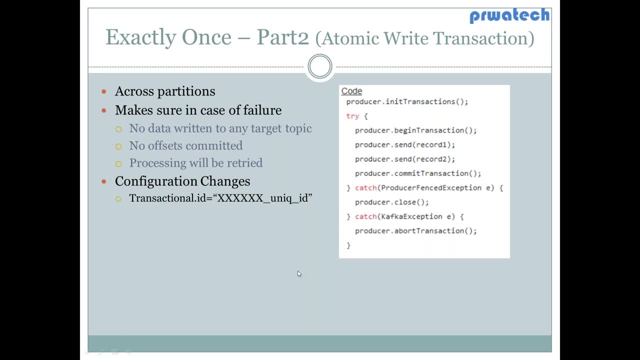 are not, uh, actually being in the particular partition, particular partition. so to resolve that we have atomic right transactions, okay, atomic means, uh, it will happen everything or nothing, everything or nothing. so when producer will send them as, so we can see this code. so producer in a transaction, producer begin transaction, then producer send. 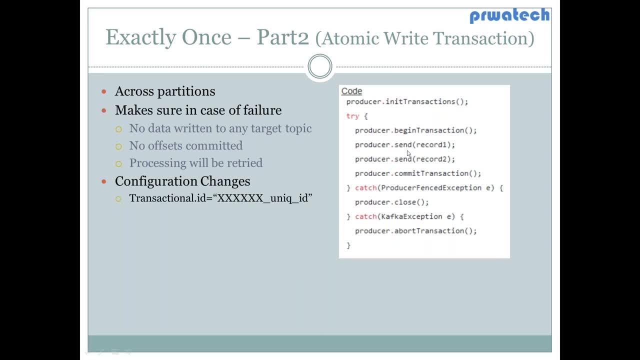 record one producer. second, send record two. all this when these two will be successful. at that time it will happen that, okay, uh, your transaction will be committed. if there is any a error, it will go to the catch block producer, will be closed or any. it will be or it will. 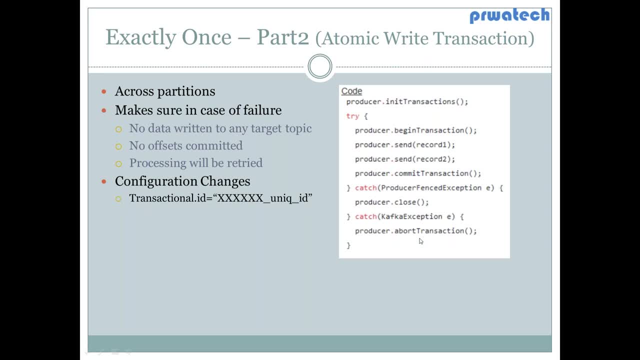 be about transaction process, okay, in the catch block. so the the kafka broker will not contain any message. if it is, if there is any fail, okay, any fail to any partition. so no data written will be written to the any target topic. no offsets will be committed process. 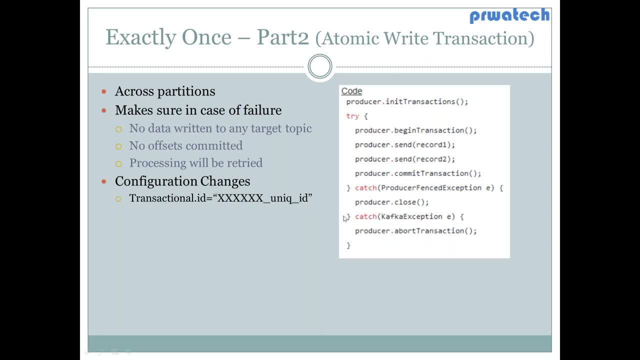 will be required so for so for to you to have this atomic transaction, you just need to have one transactional ID. okay, any number, and then you have. you can have any unique ID using the transactional ID. it will check for each transaction. it will have one transaction. 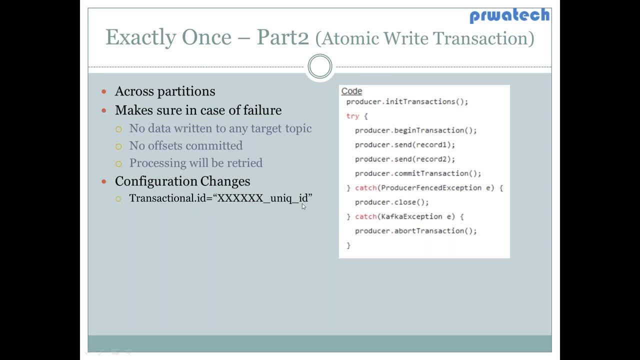 unique transaction ID. okay, it will generate one unit transaction ID and that that will make sure that your transaction as a whole is success or not. if it is fail, then nothing of your data is being persisted to kafka. okay, so till now we have handled producer and kafka level. now let's go to the consumer level, because it's 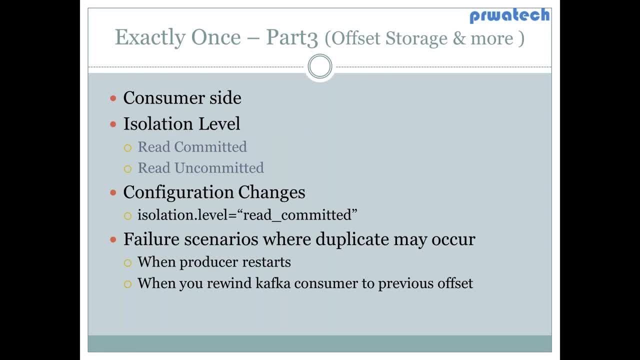 an end-to-end process. now, at the consumer level, what happens is that there is one. there are two kinds of offsets. you can read consumer, consumer can read read committed and read uncommitted. read committed means your producer sends message to the kafka and then the consumer power uses the literal or the kings aprendices and satirize, send message to the consumer. 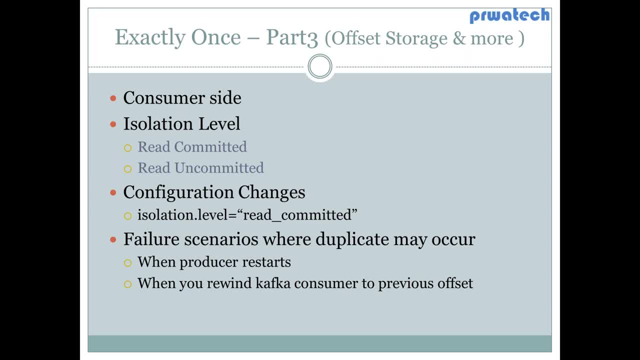 when the customer posts message to the user or their négociations to the user, it may be style Shiny, your messages are being committed to. each partition meant like the. your data is in sync. okay, so if your data is in sync, that means your data is actually persisted once in kafka. 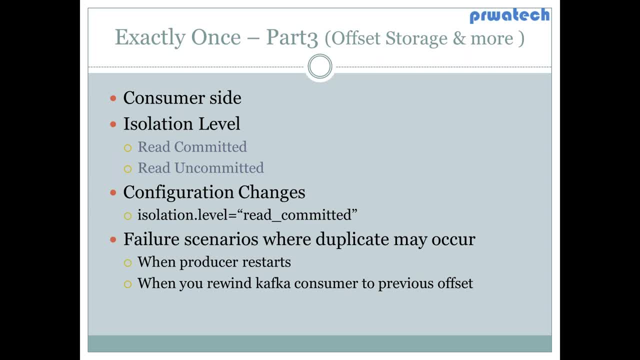 broker and its insync. every, every broker has that, so you will. i will call it read committed. read uncommitted means there is some problem. it's not an insync, okay. so if you have your isolation level read committed, your consumer will answer that question before you drop for a wounds. you will be reaching these options multiple levels. it is going to appear in your rendition thing when so on. so when we haveups where the login password has to enable extract further, do this in ref scripture. so rempli's not put. uh no, the ing took step code in the afternoon. 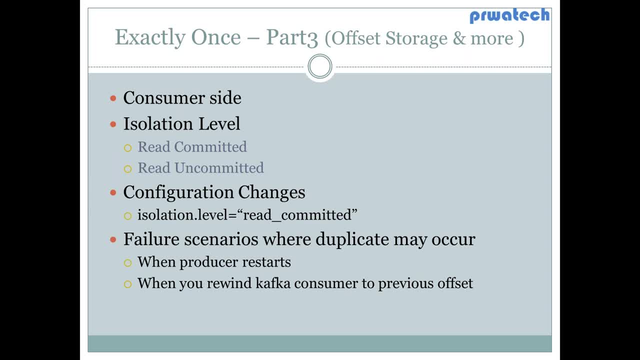 this will be at the consumer level. okay, so your consumer will only able to read, only for which are read committed, and Kafka will all. as I said before, the Kafka already till for so far maintains that. okay, there will be one copy of that record, only one once. so this is how, end to end, from producer side, Kafka side, and 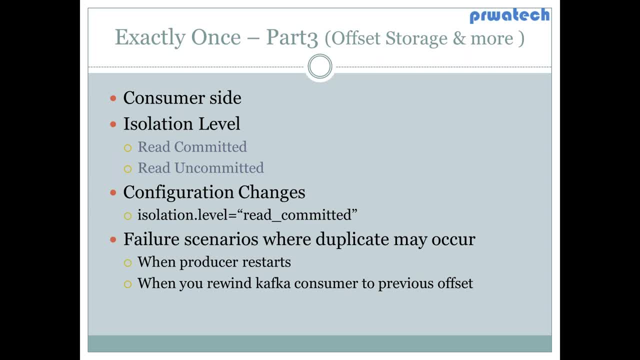 then for is a consumer side is exactly one. semantics is maintained. now there is will be failure scenario, like when producer restarts. producer restarts means producer ID is different. producer ID is different means. it won't be tough. I won't be able to recognize that it's the same message or different message. 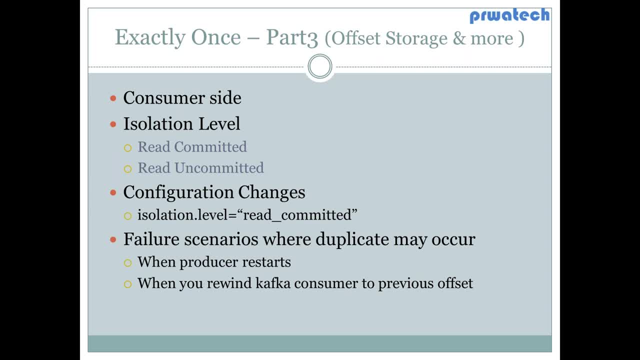 the sequence number is same but producer ID is different, so in that case it will process the data again. there will be duplication. this is one scenario which is an edge case, but yes, these are some scenarios. when you rewind your Kafka consumer to previous offset, this is your use case. 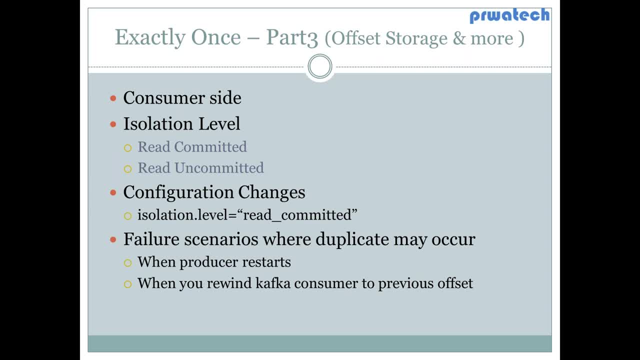 you are specific. actually, sometimes we need to consume data again from the consumer side. okay, we need to consume that. we consume once and there is some problem and we need to really consume that. at that time we need to rewind your Kafka consumer and this offsets right in in the of these offsets are present in your 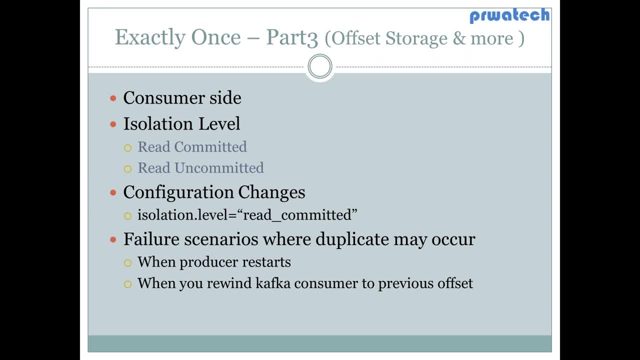 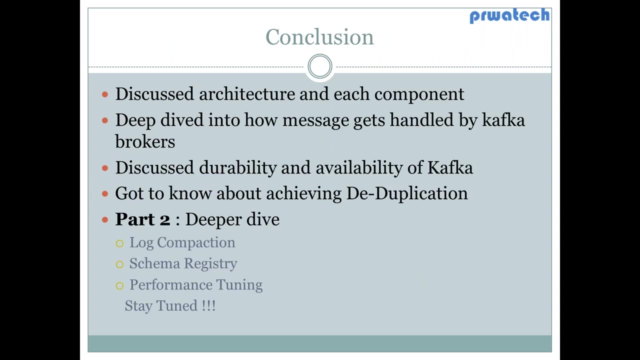 partition. now consumer controls the reading of the offset. so it can go, it can rewind it when it can forward, like this, so it can rewind. so consumer has the control. so if it wants to read the message, then it will read the next. Ok, so this conclusion is that 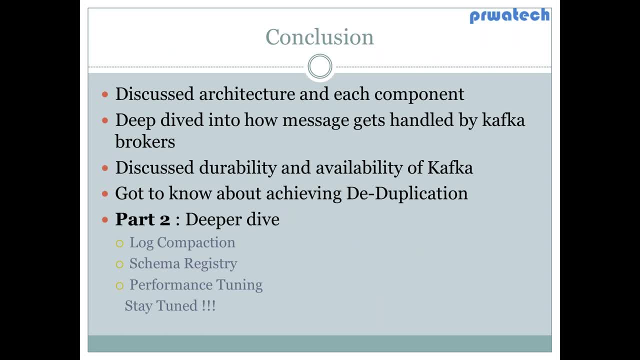 so we have discussed this architecture and each. so we have. we have discussed each architecture, its component of that, and we talked about it. so, over details, I think these has been very useful, so thank you very much. so let's go to certain we have been typed into how message gets handled. 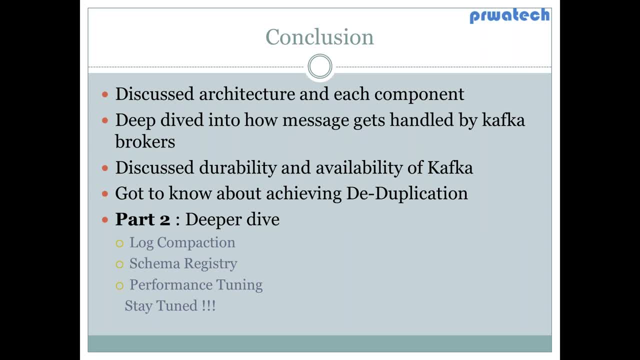 by Kafka broker That we went to detail how message are actually being into the, how producer is sending the message, how in the partition in the broker, in the broker. there will be topic inside that partitions, multiple partitions, replication factor. 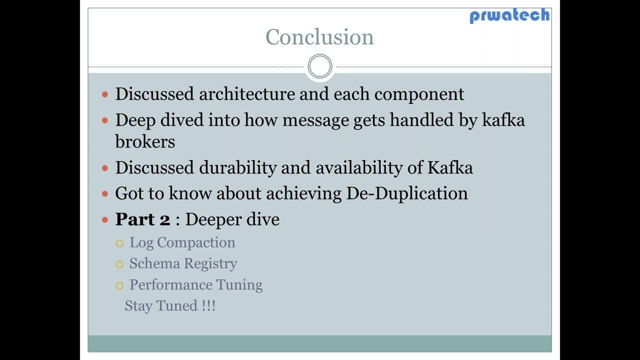 We all discuss that And we also discuss the durability available to Kafka. That means your replication, how your leader, follower, controller. if one leader gets failed, then what happens? How controller manage everything. If your controller also goes down, it will take a bit time because Zookeeper has to check some. 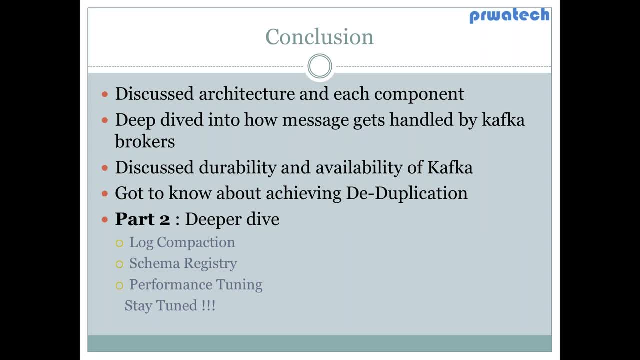 which broker is in sync and whichever interest condition which will create the controller directory passed in the Zookeeper directory at that time, that will be the controller. So and also we discussed about exactly one semantics, that is, deduplication of the message from end to end. 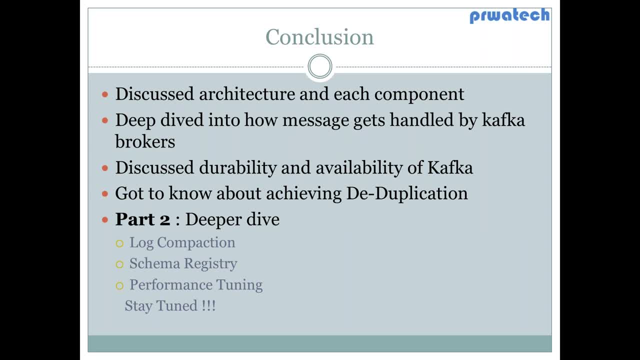 That is from producer Kafka and the consumer. Okay, so this is for the first part And there will be more to discuss, but in one hour, very less time. So I have put one second part. please stay tuned There. we can discuss more on log compaction. 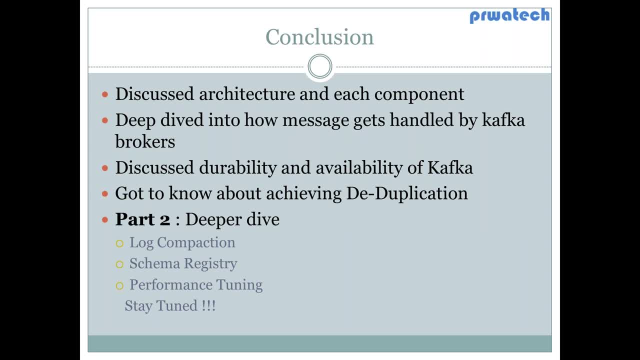 schema, registry, performance tuning, all those advanced topics. Okay, there will be another conceptual right statement. Thank you very much. Any questions, please? Okay, so there are a few questions. Don't we get consumer at the end? That I discussed already.